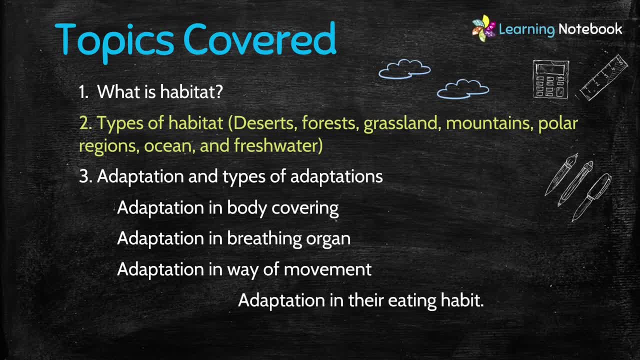 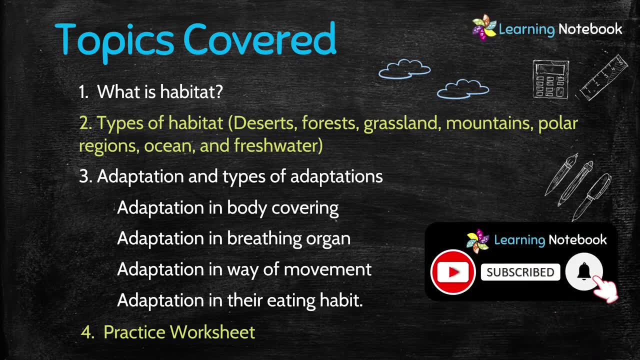 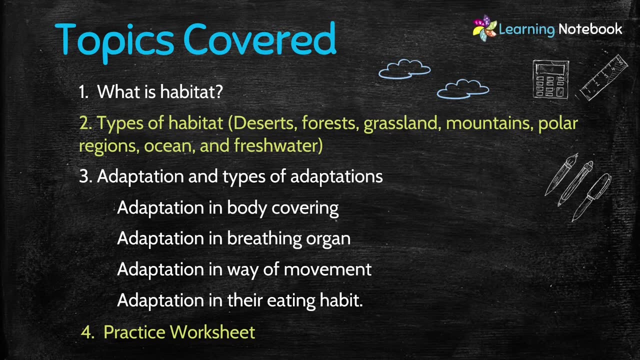 what is habitat? Then we will learn types of habitat, ie deserts, forests, grassland, mountains, polar regions, ocean and fresh water. After that we will learn adaptation and types of adaptations, ie adaptation in the habitat. So let's start. 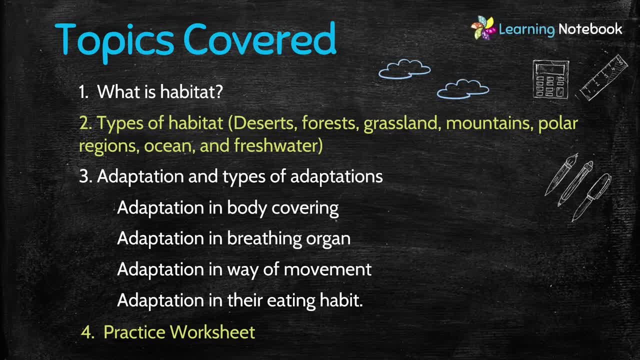 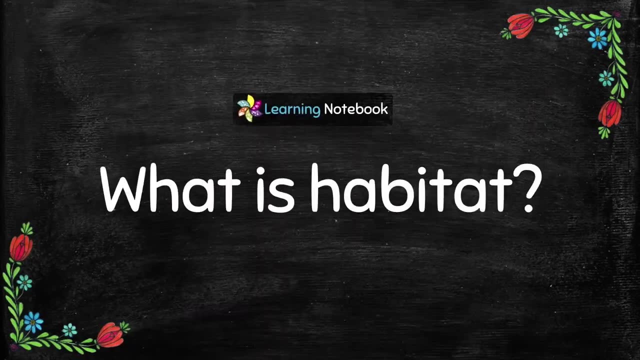 Adaptation in body covering, adaptation in breathing organ, adaptation in way of movement, adaptation in their eating habit And students. in the end, I will also give you a worksheet for your practice. So let's start and first learn what is habitat. 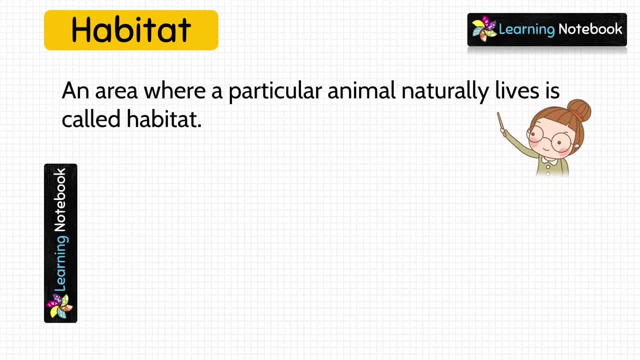 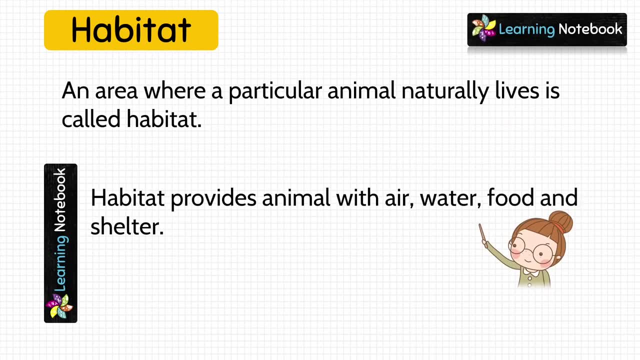 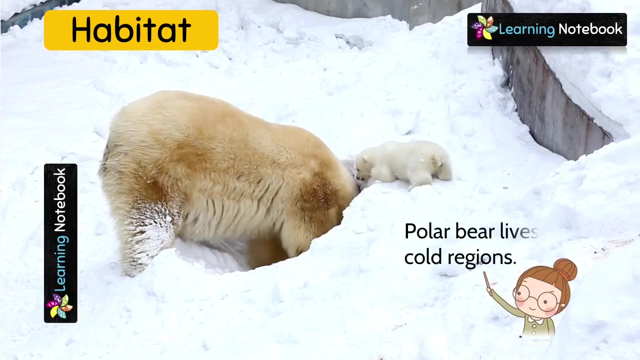 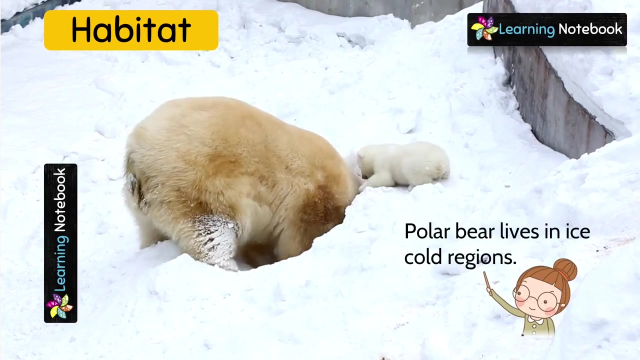 An area where a particular animal naturally lives is called habitat Habitat, And a habitat provides animal with air, water, food and shelter. Let's understand habitat with the help of few examples. A polar bear lives naturally in ice-cold regions, So ice-cold region is a habitat of polar bear. 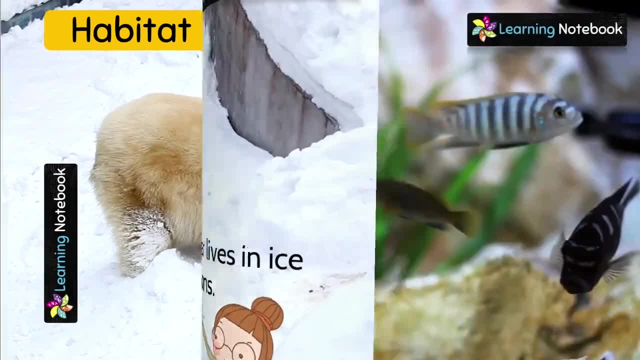 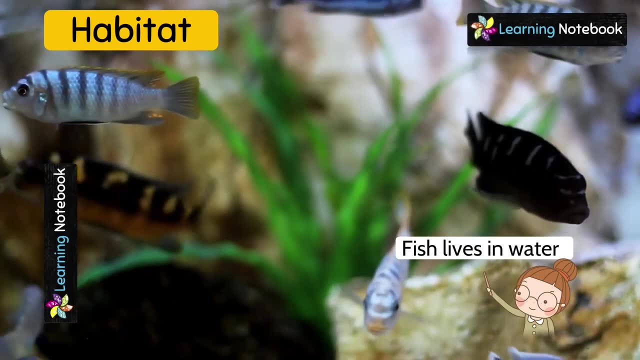 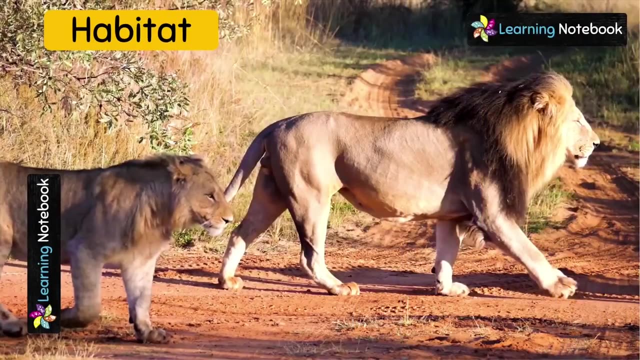 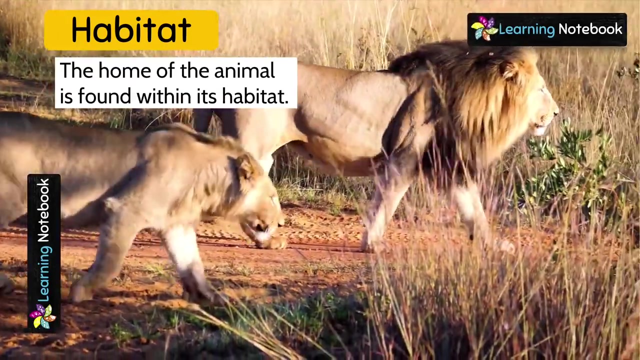 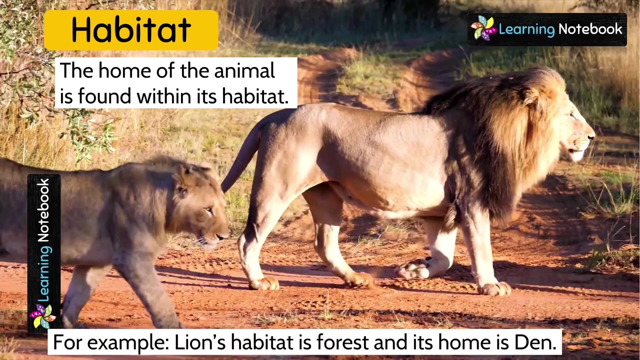 Water. Fish lives in water, So a water body is the habitat of a fish. The home of the animal is found within its habitat. For example, lion's habitat is found within its habitat That is forest, And its home is den, which is in the forest. So the home of the animal is found within its habitat. 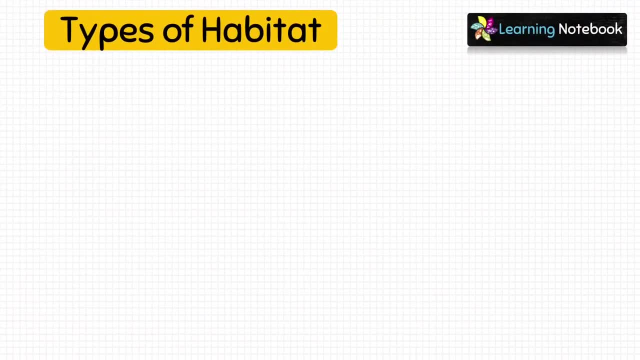 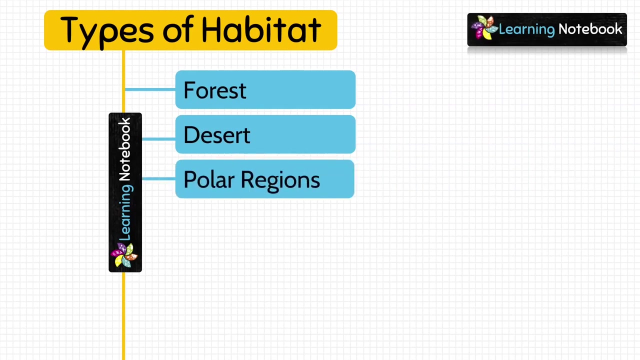 There are different types of habitat on earth. They are forest, desert, desert and desert. There are different types of habitat on earth. They are forest, desert, desert and desert. Polar regions. Ocean Freshwater, which includes ponds, rivers and lakes. 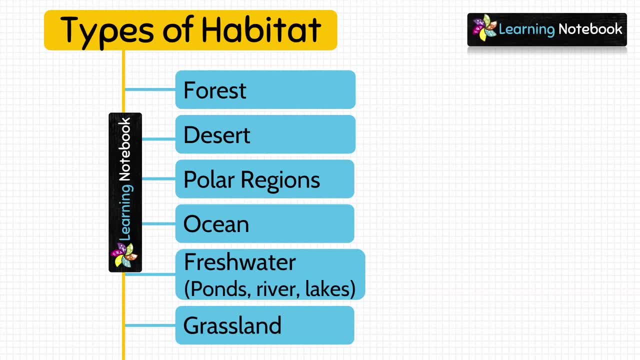 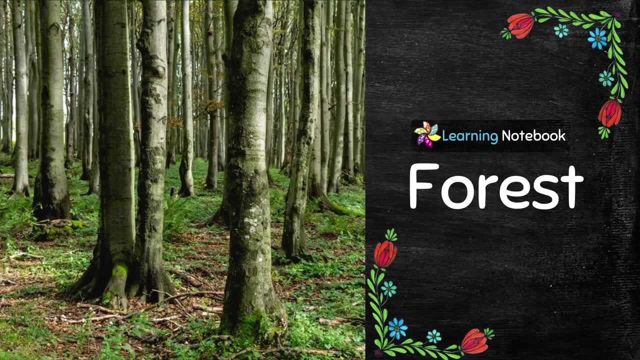 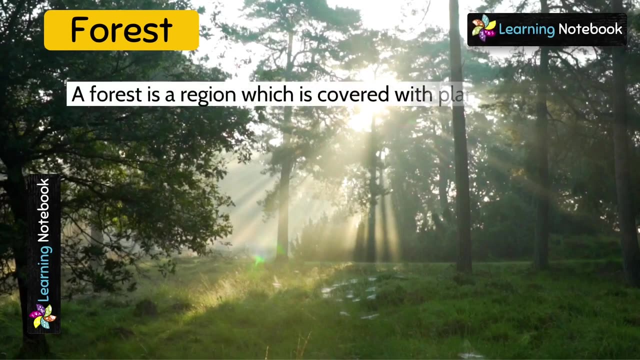 And then grass land. Let's understand them one by one. First type of habitat is Forest. A forest is a region which is covered with moderate cantidad of newcomers, A region of the HOLY. GDP is around 40,000 acres of land per acre. 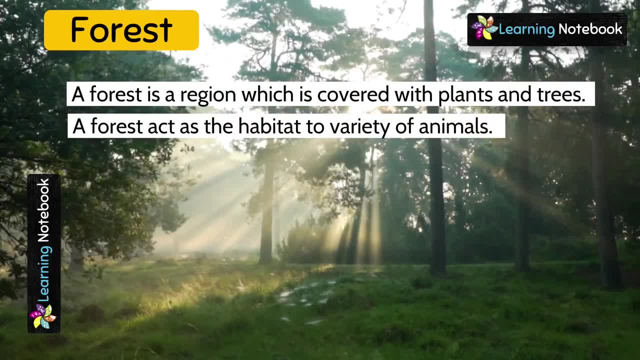 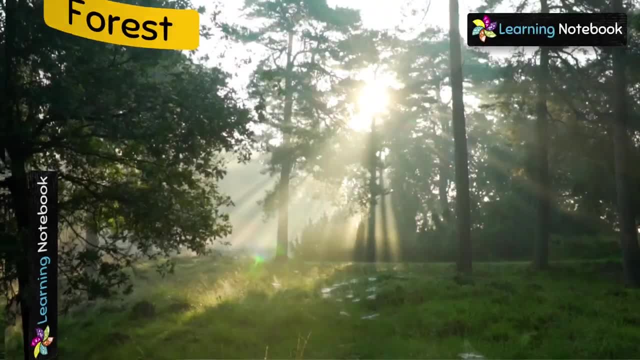 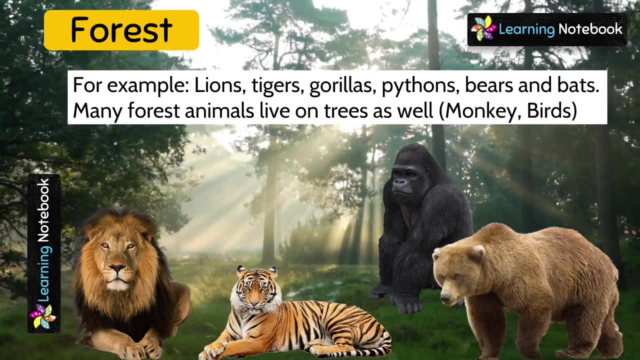 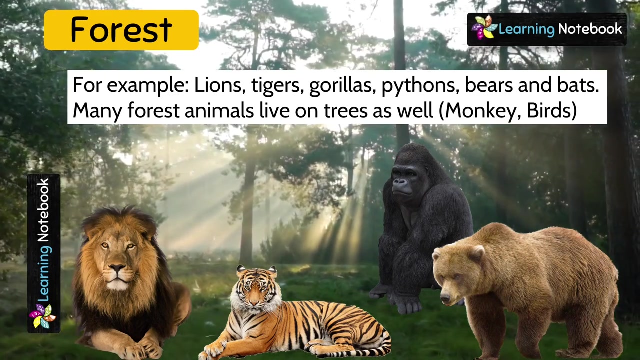 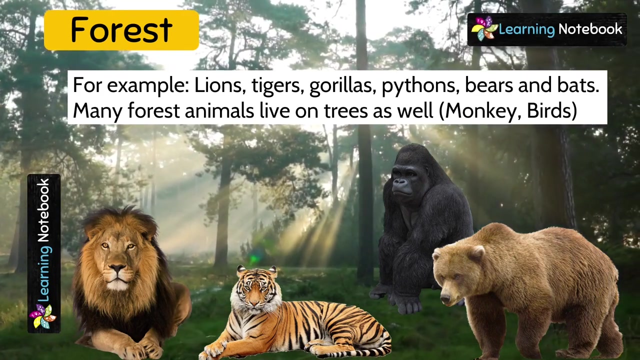 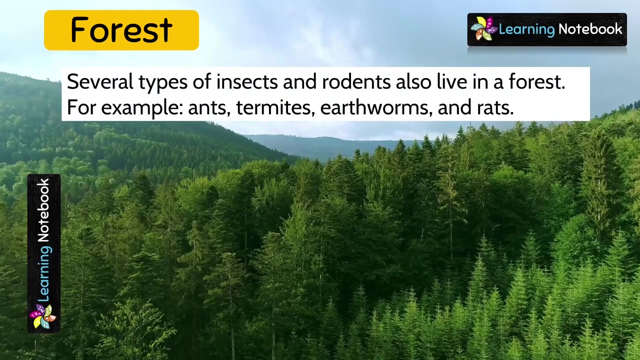 with plants and trees, and a forest act as the habitat to variety of animals, for example lions, tigers, gorillas, pythons, bears, bats. all of them live in forest, and many forest animals live on trees as well, like monkey birds, langur's. also. several types of insects and rodents also live in a forest for. 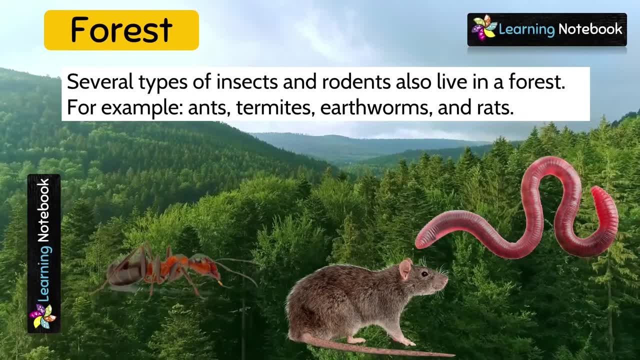 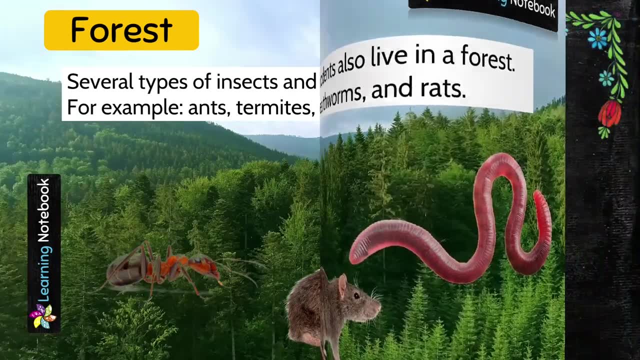 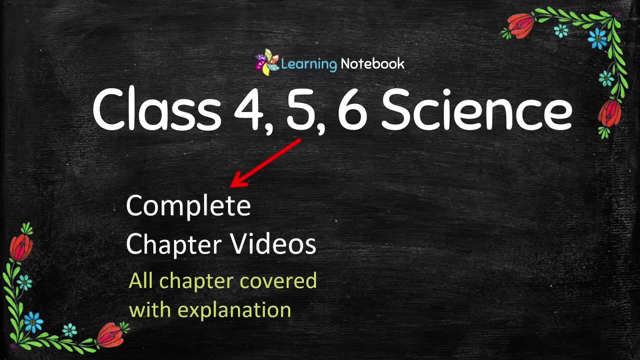 example, ants, termites, earthworms and bats, so some of these animals are able to live in the forest also. several types of insects and rodents also live in the forest, for example, ants, termites, earthworms and bats. They also live in a forest. Students, we would like to tell you that we have made videos on every chapter of class 4,, class 5 and class 6 science. 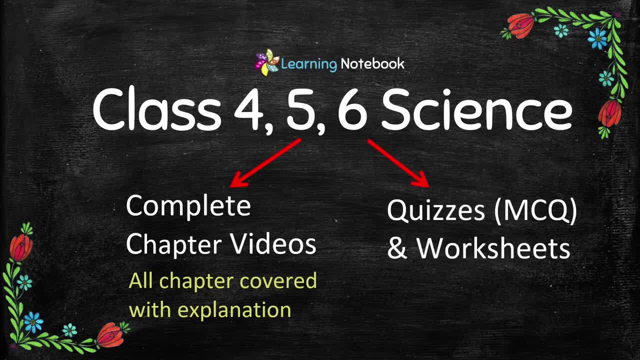 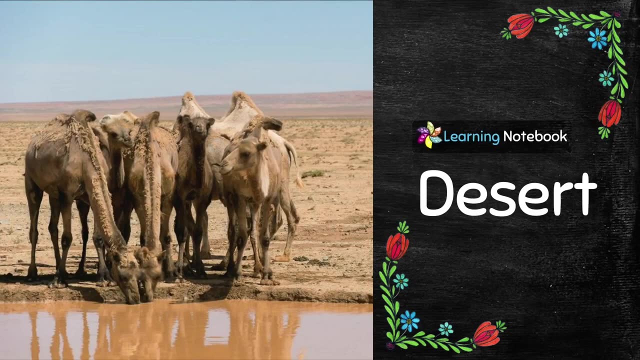 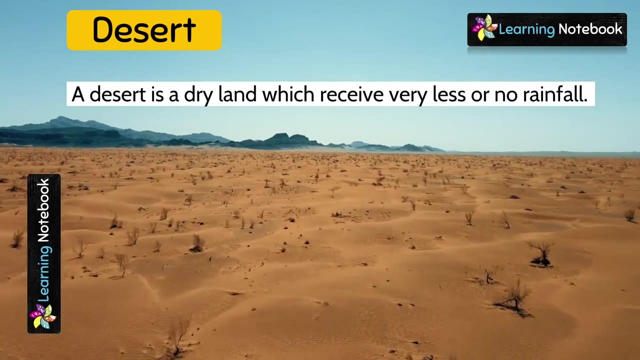 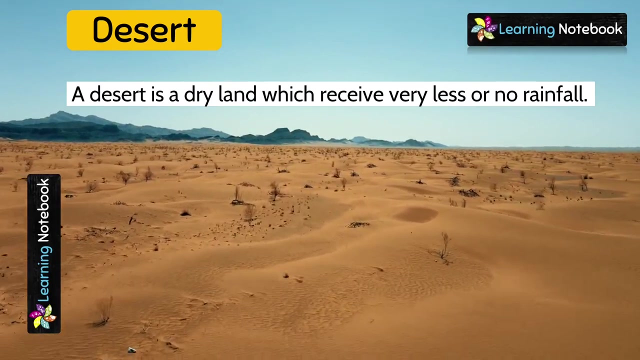 We also have interesting worksheets and quizzes on each chapter, So I would suggest you to check out our channel Learning Notebook Now. next move to next type of habitat: desert Students. as you can see here, a desert is a dry land and it receives very less or no rain fall. 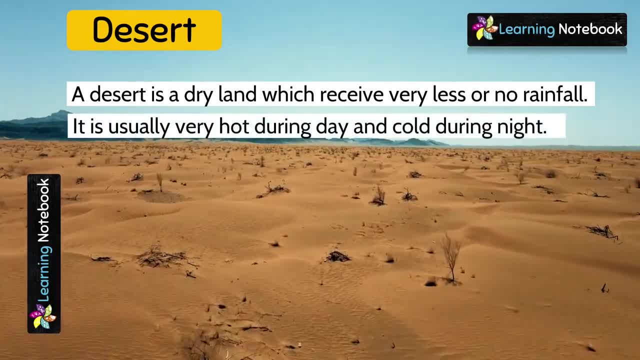 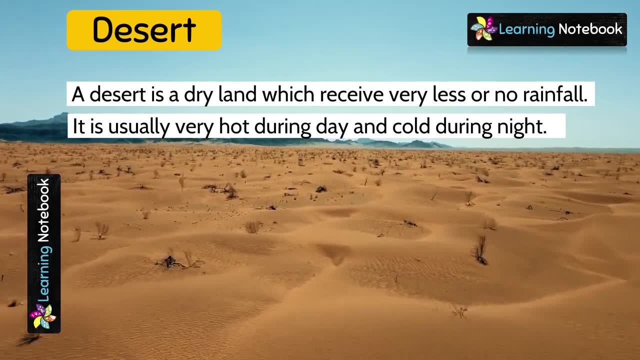 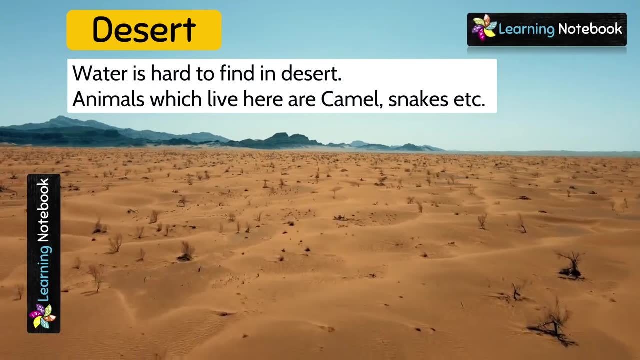 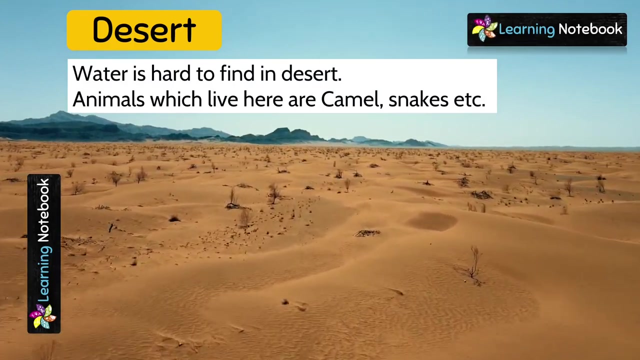 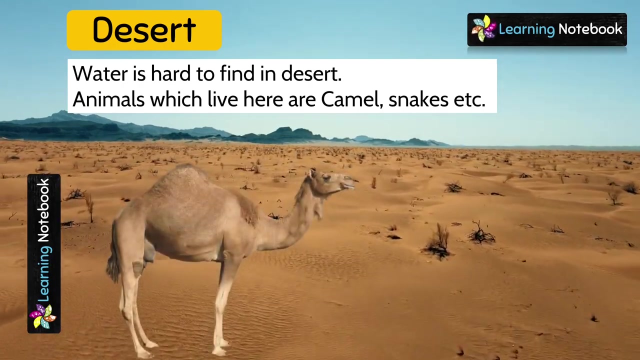 It is usually very hot during day And cold during night. Water is very hard to find in desert. Therefore, only those animals which can survive using less water are found in desert, Like camel and snakes. They are found in desert because they can survive on very less water. 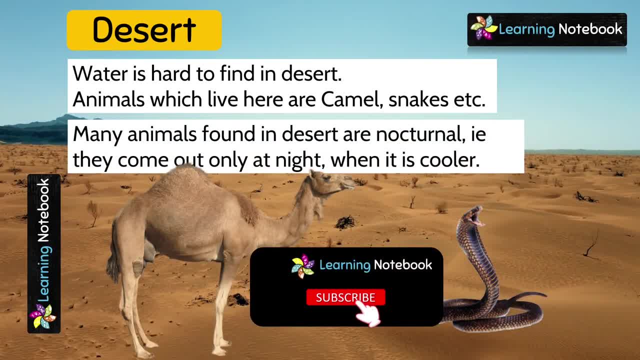 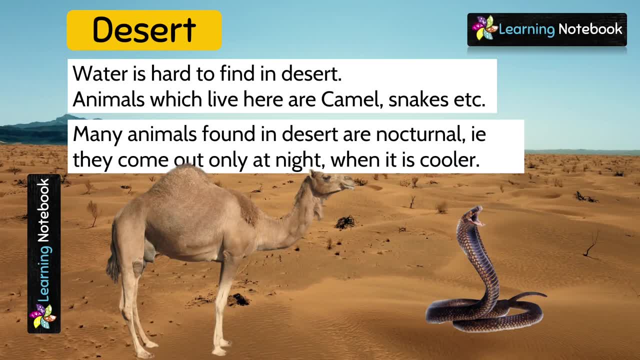 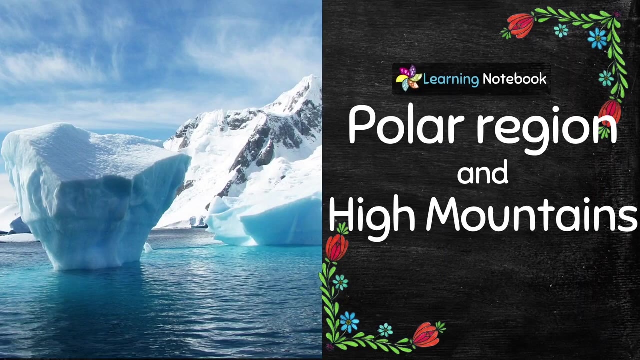 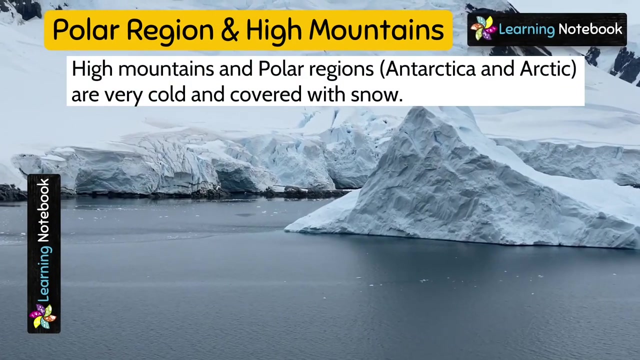 And many animals found in desert are nocturnal, That is, they come out only at night, when it is cooler, And they spend rest of their time underground. Now next type of habitat is polar region and high mountains. High mountains and polar regions. 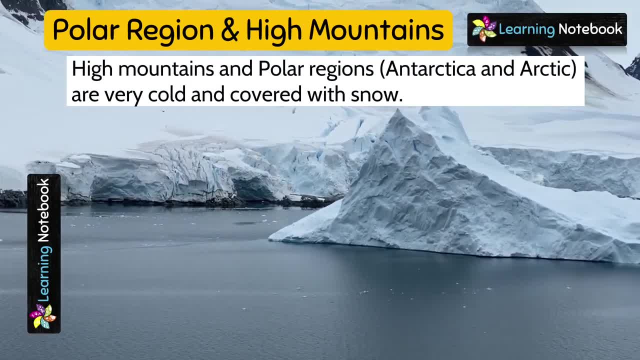 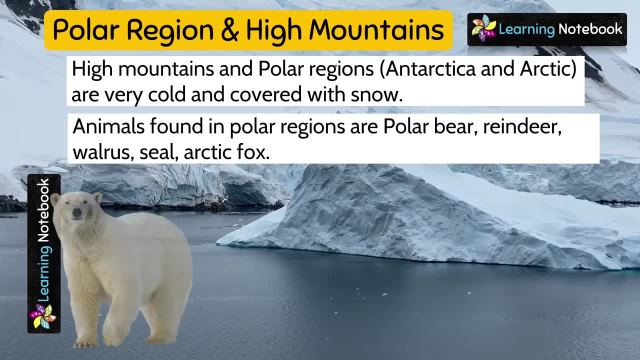 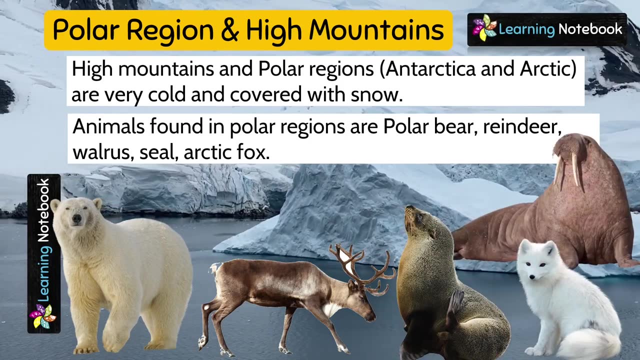 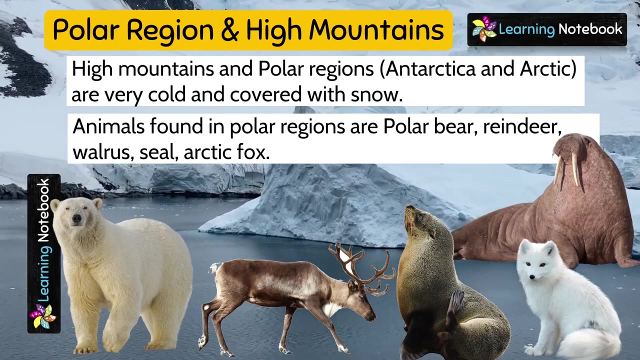 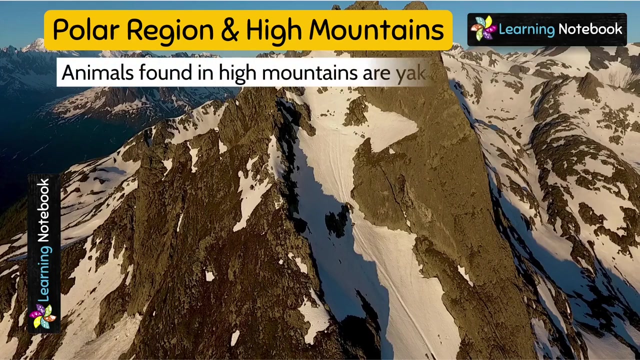 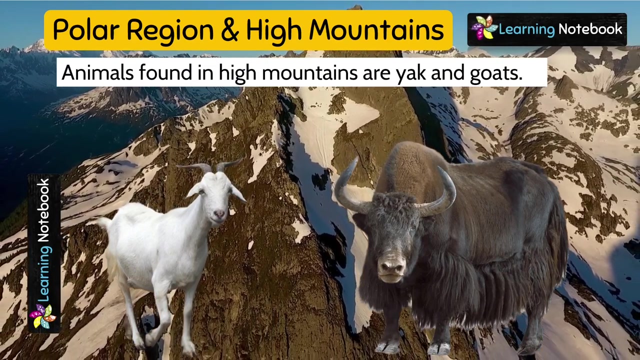 Polar regions include Antarctica and Arctic. These are very cold and they remain covered with snow almost all the year round, And animals found in polar regions are polar bear, reindeer, walrus, seal, arctic fox. Both polar regions and high mountains are among the coldest and most harsh habitats. 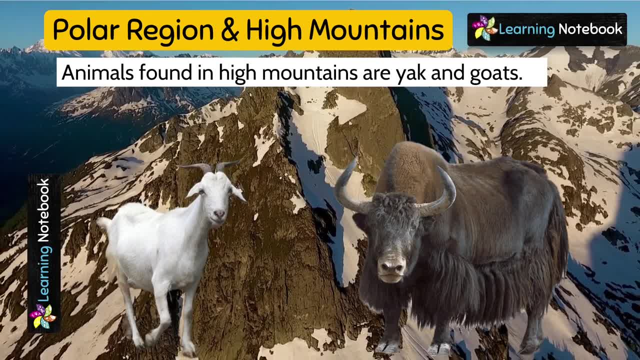 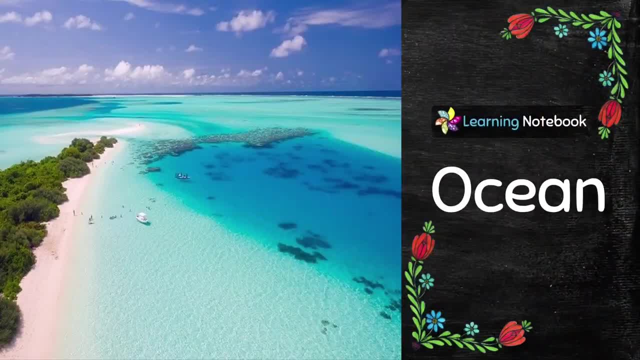 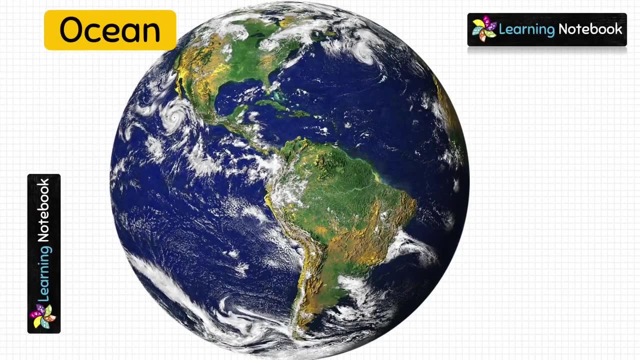 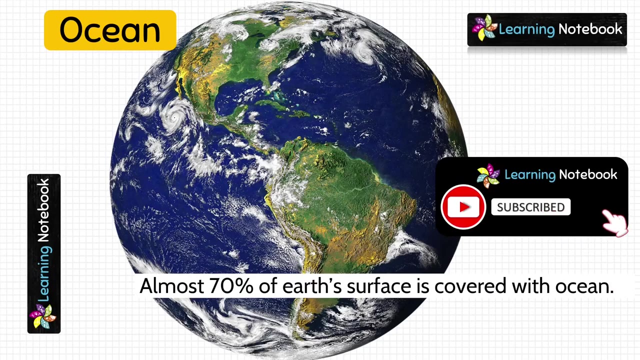 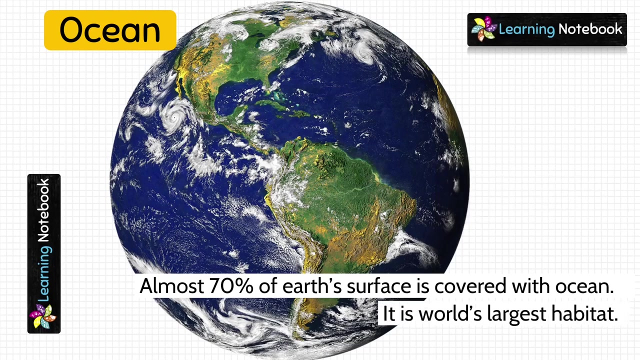 And some of the animals found in high mountains are yaks and goats. Now let's learn about next type of habitat, which is ocean. Almost 70% of the earth's surface is covered with ocean And therefore we can say ocean is the world's largest habitat. 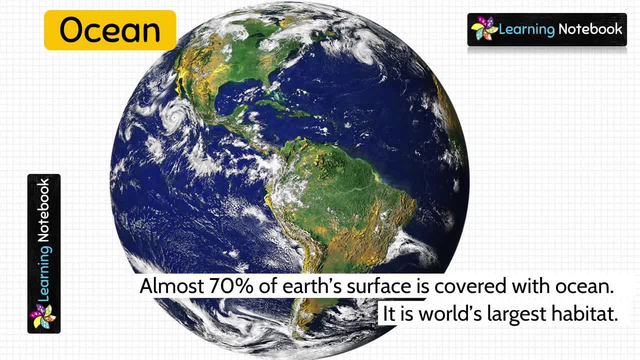 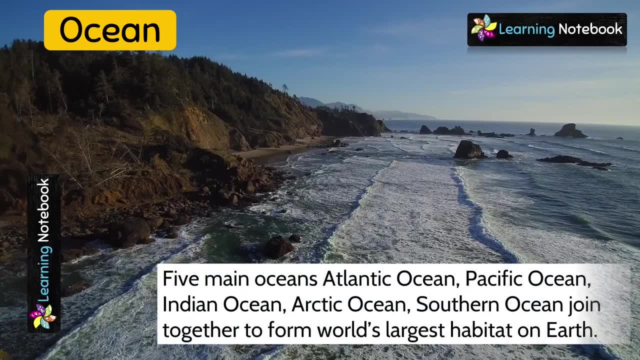 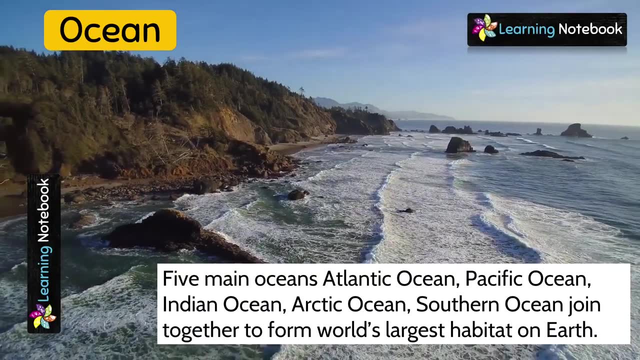 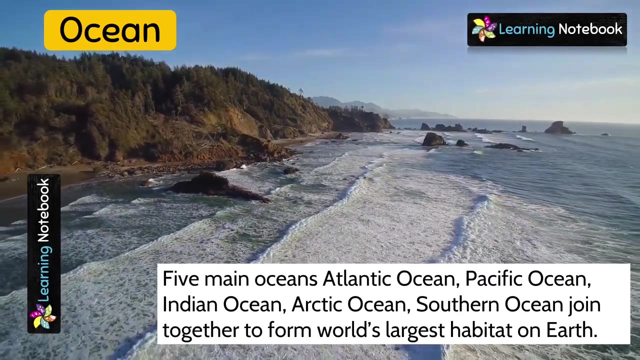 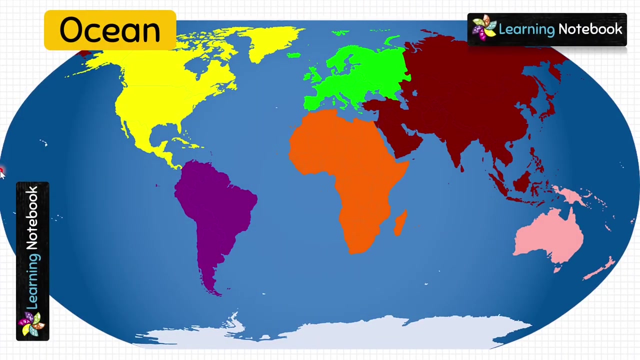 Ocean water is salty and is also known as marine habitat. 5 main oceans- Atlantic Ocean, Pacific Ocean, Indian Ocean, Arctic Ocean and Southern Ocean- join together to form world's largest habitat on earth. Now, students, let's see where these 5 oceans are located on our earth. 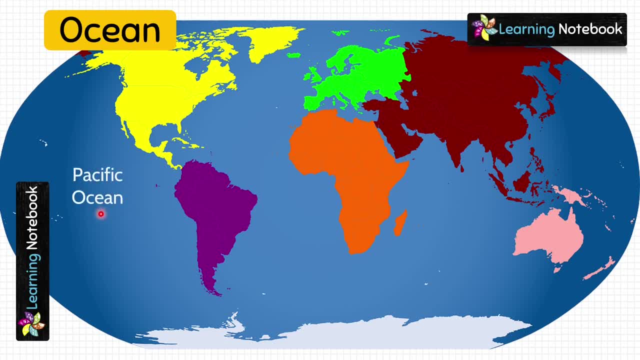 Here we have Pacific Ocean, Then here there lies Atlantic Ocean, Then below India we have Indian Ocean, And on the top we have Arctic Ocean And here we have Southern Ocean. So these 5 oceans together form the largest habitat on earth. 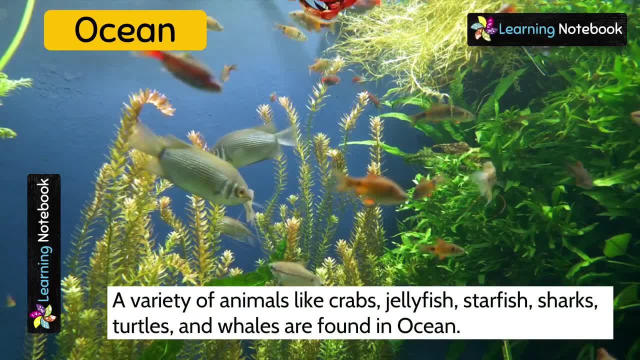 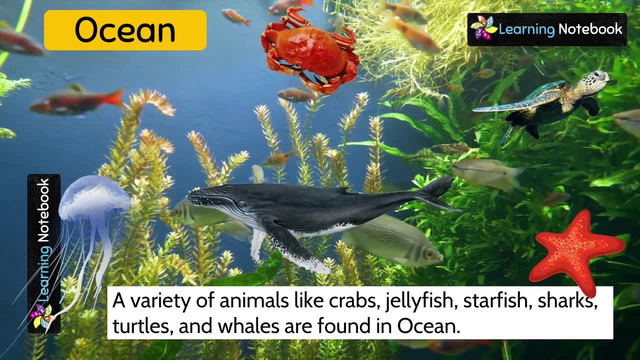 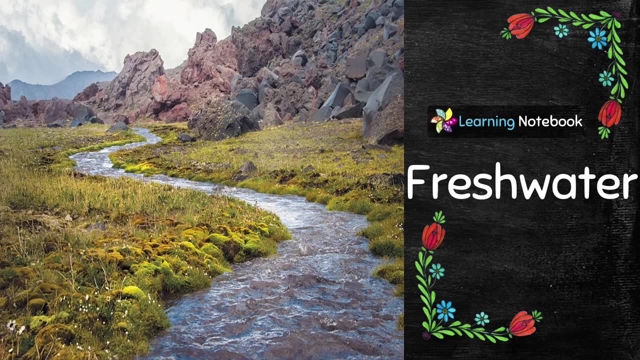 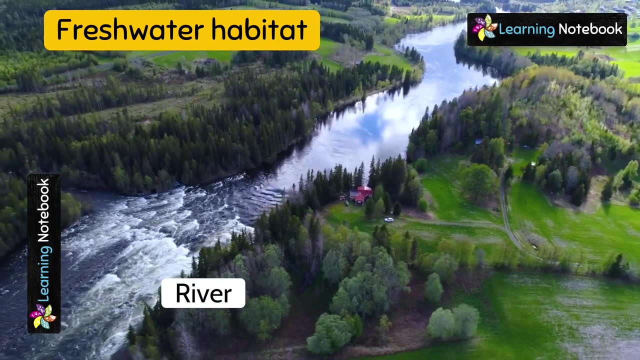 A variety of animals like crabs, jellyfish, starfish, sharks, turtles and whales are found in ocean. Next type of habitat is fresh water. Let's see sources of fresh water River- This is a river. This is a river. 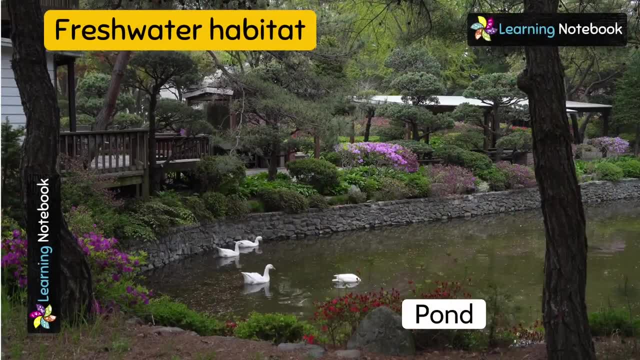 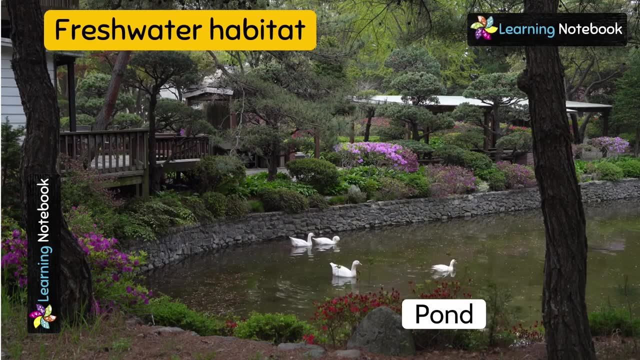 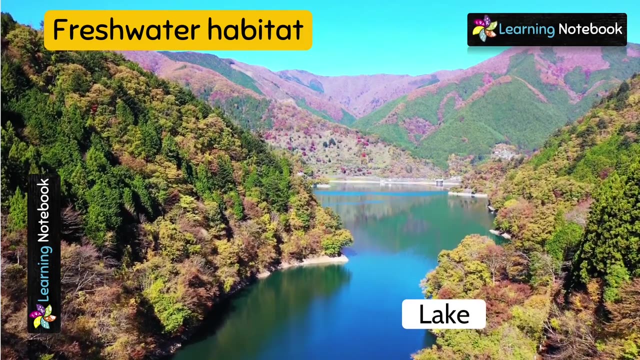 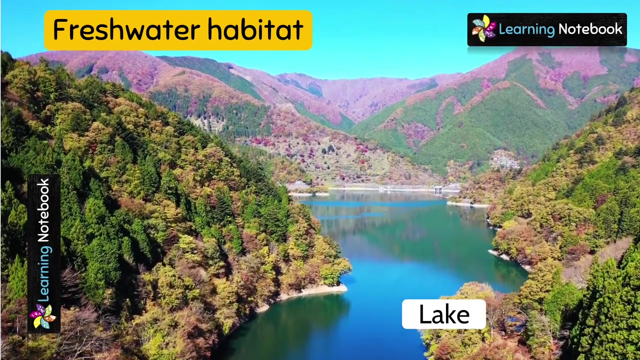 This is a tunnel. This is a pond. Next source is fountains. Another source is ponds. Next source is ponds. We have lakes. Lakes are sources of fresh water, Boundaries of fresh water, Places used in the urban above us. 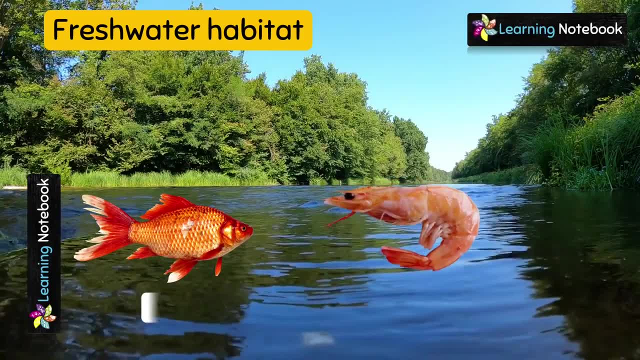 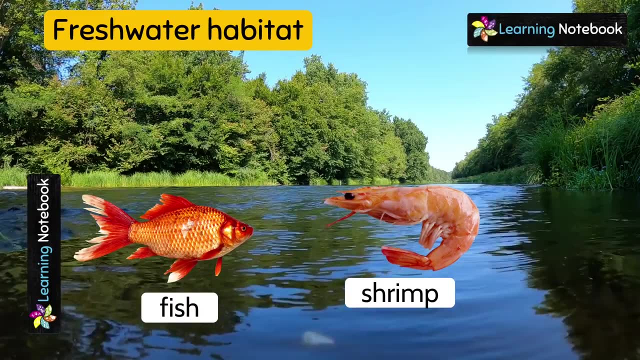 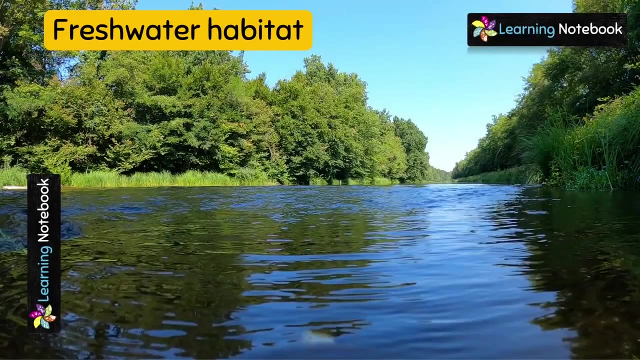 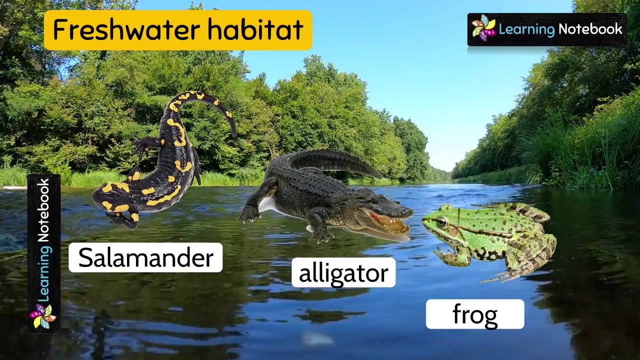 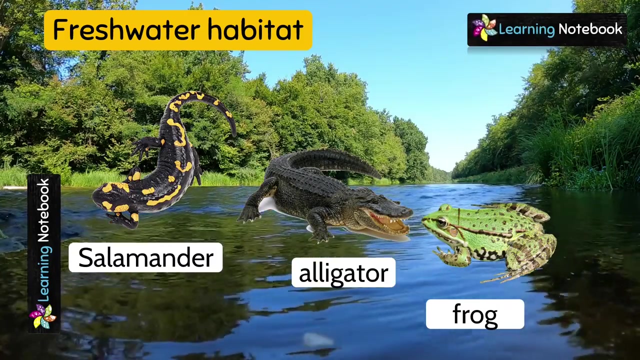 Lakes. Fresh water is a habitat to many animals like fish and shrimp, but these animals can live in water only. There are other animals like salamander, alligator, frog, crocodile, which also live in fresh water, but they can live in water as well as on land. 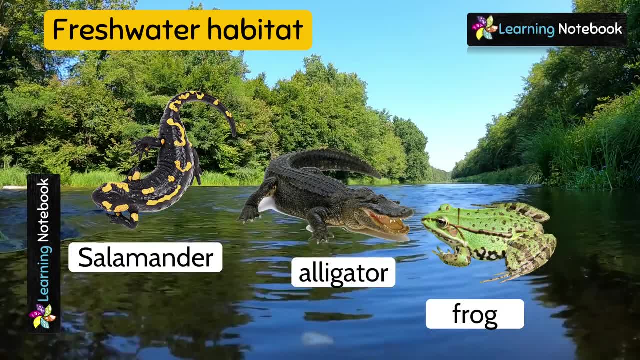 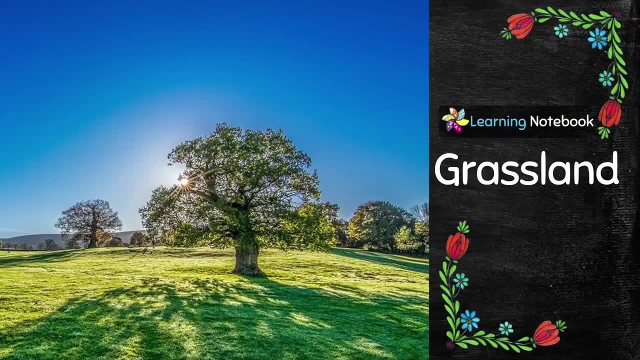 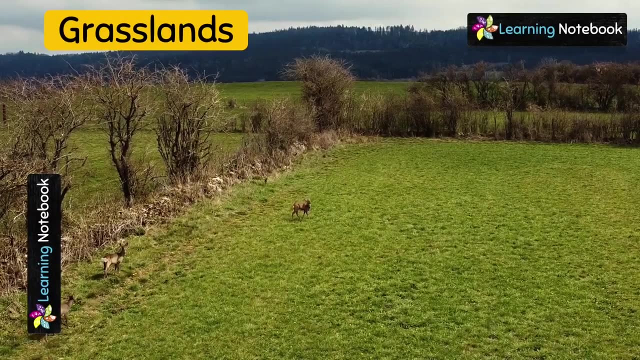 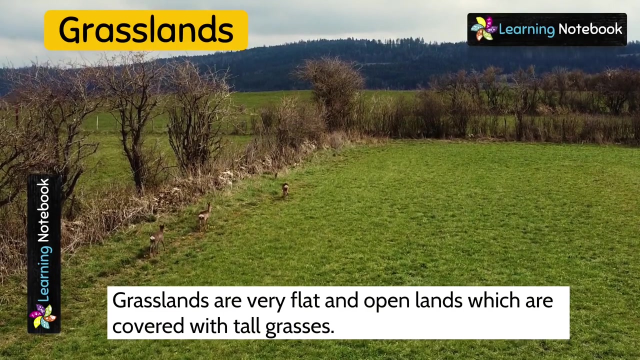 Students. do you know what such animals are called as? Do tell me in the comments box. Now, our last type of habitat is grassland. So what are grasslands? Grasslands are very flat and flat. They are open lands which are covered with tall grasses. 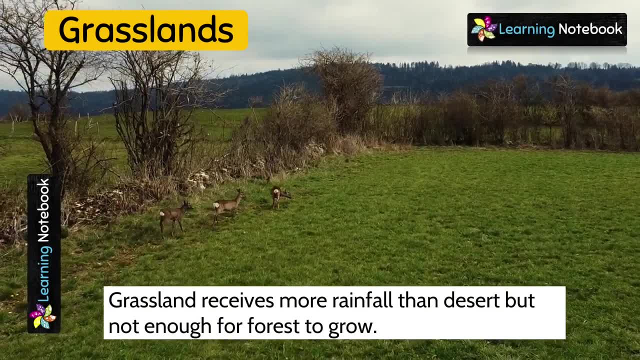 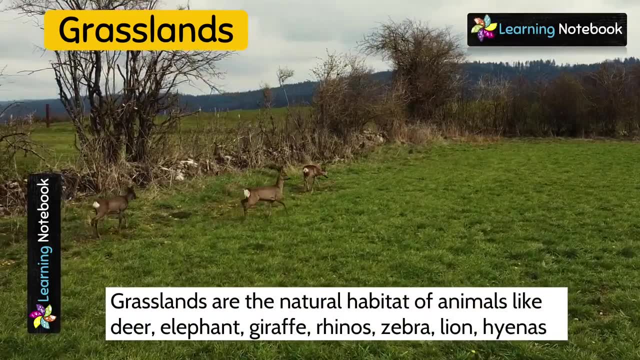 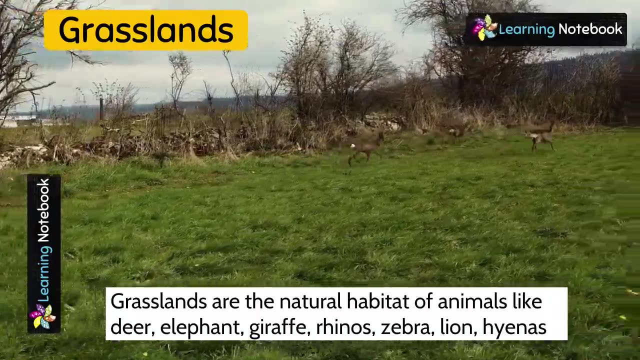 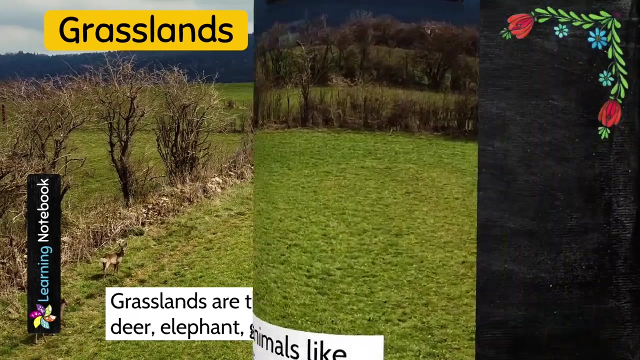 They receive more rainfall than a desert, but not enough for a forest to grow. Grasslands serve as a natural habitat for animals like deer, elephant, giraffe, rhinos, zebra, lion and hyenas. So what are grasslands? Grasslands are the natural habitat for sheep. 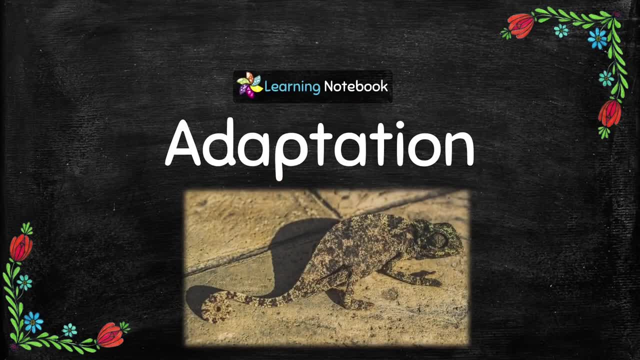 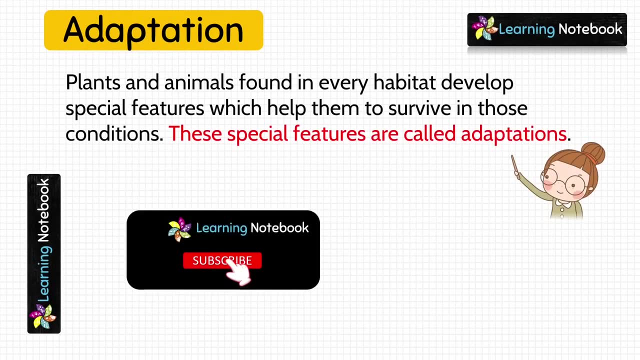 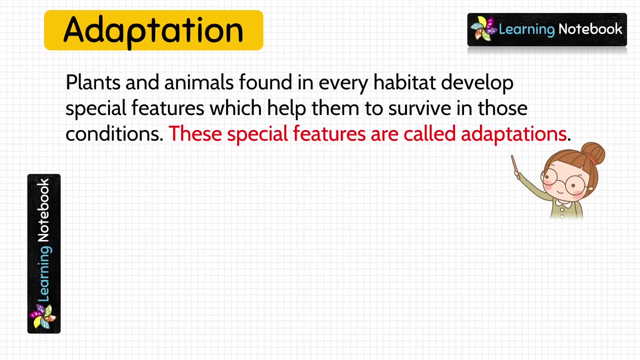 Now let's move to our next topic, which is adaptation. So first let's understand what is adaptation. Plants and animals found in every habitat develop special features which help them to survive in those conditions, So these special features are called adaptation Students. in this chapter we will study only about adaptation of animals. 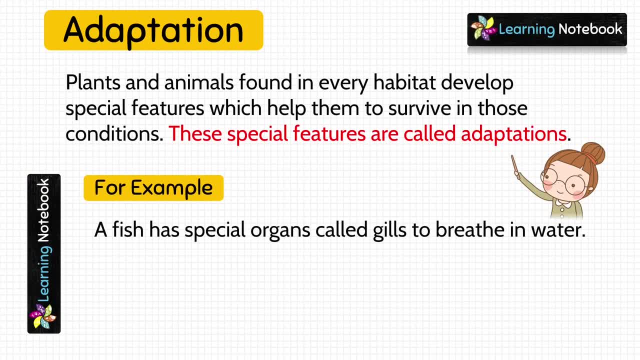 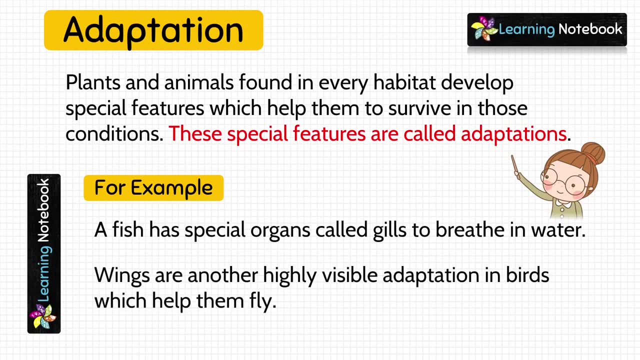 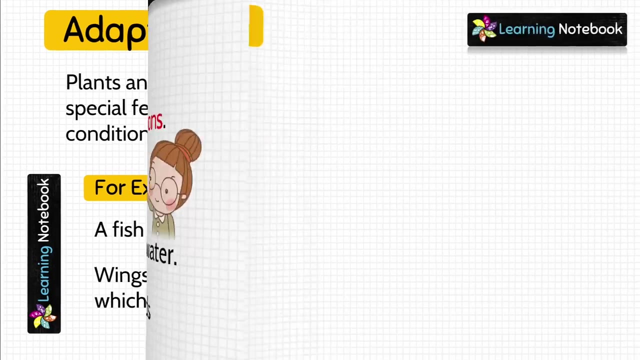 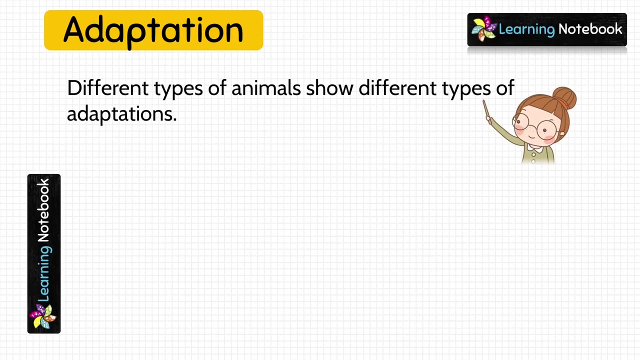 See some examples of adaptation A fish. A fish has special organs called gills Which help it to breathe in water. Wings are another highly visible adaptation in birds, Which help them to fly. Different types of animals show different types of adaptations. Adaptations may be in their body, covering breathing organ, way of movement or way of their eating habit. 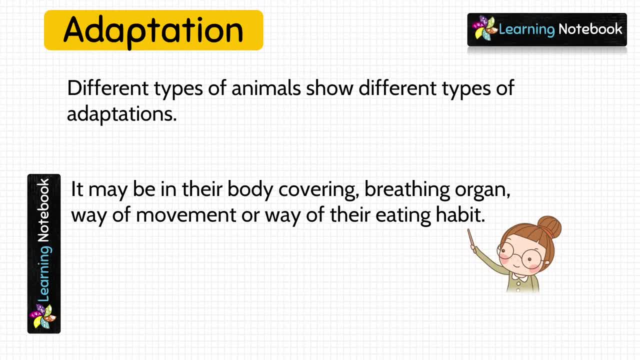 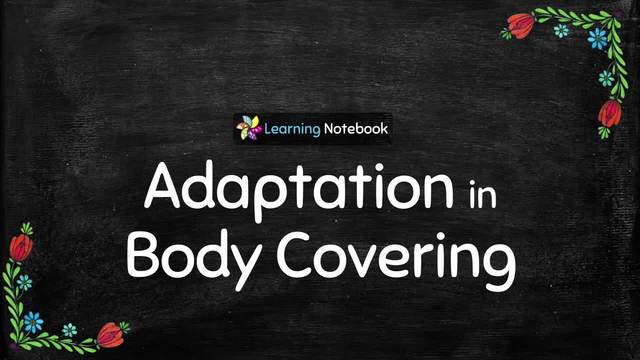 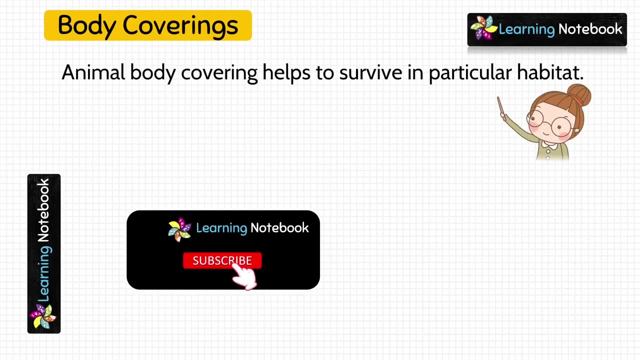 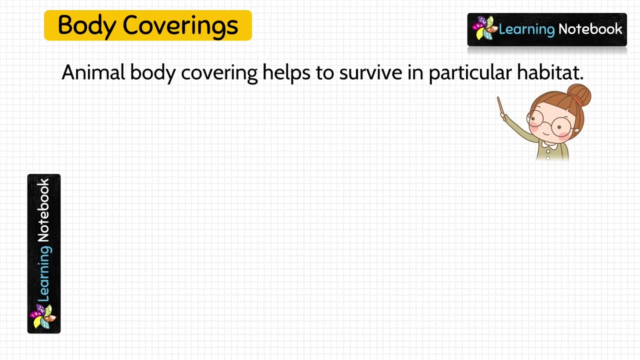 Let's learn these types of adaptations one by one. First let's learn about the body. First let's learn about the body. Let's understand adaptation in their body covering. Animal body covering helps them to survive in particular habitat. So, depending on their habitat, animals have special body coverings. 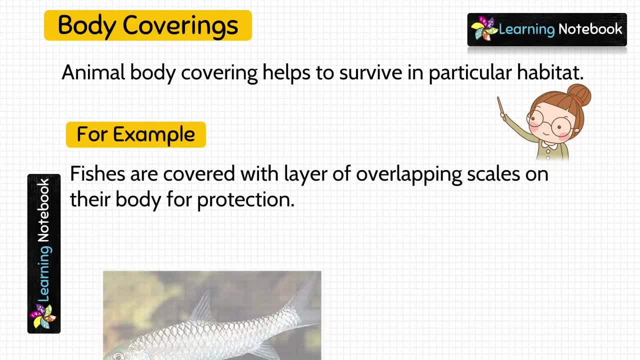 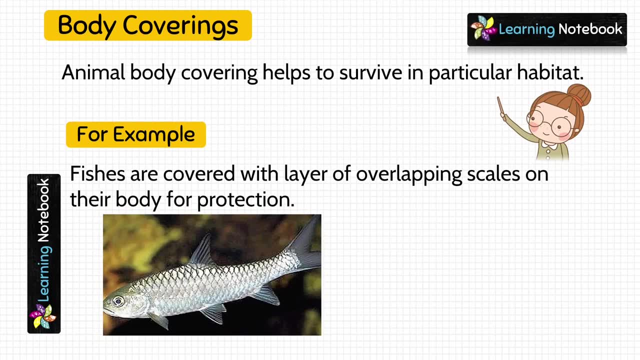 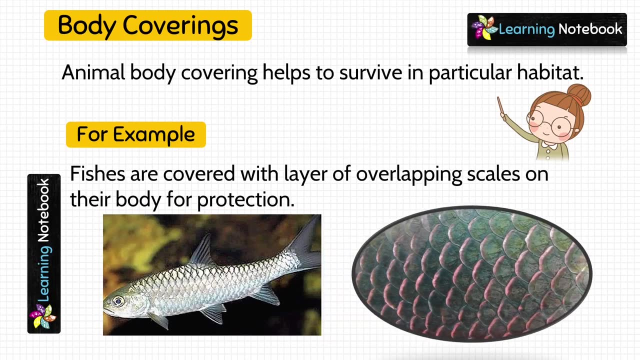 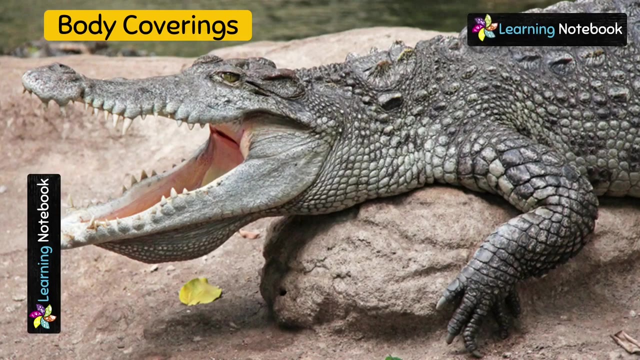 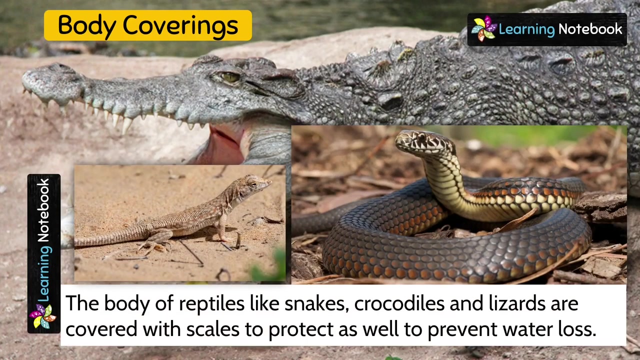 Let's see some examples. As you can see here, these are layer of overlapping scales on the fish. Let's see more examples. The body of reptiles like snakes, crocodiles and lizards Are also covered with scales to protect as well as to prevent loss of water. 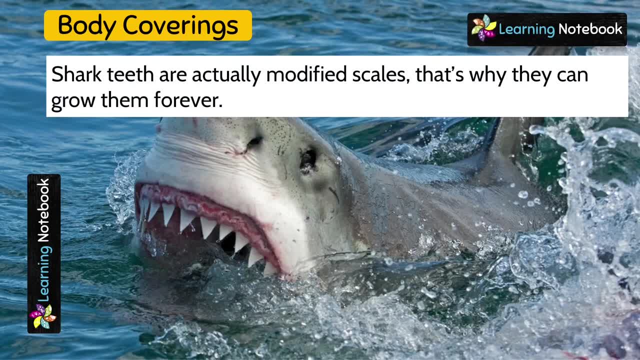 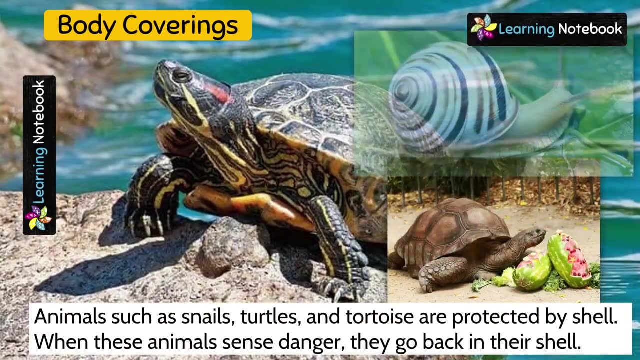 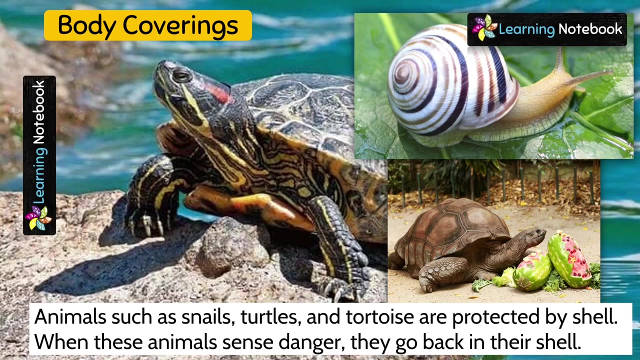 And students. do you know? shark teeth are actually modified scales And that is why they can grow them forever. Next, animals such as snails, Turtles, tortoise. They are protected by shell. Whenever these animals sense danger, they go back in their shell. 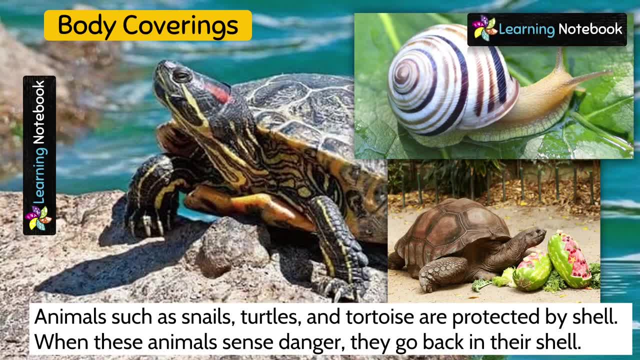 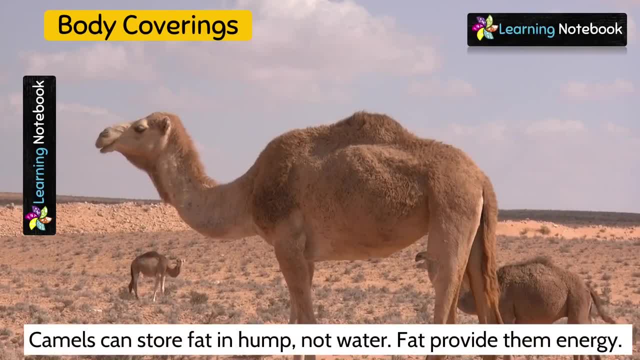 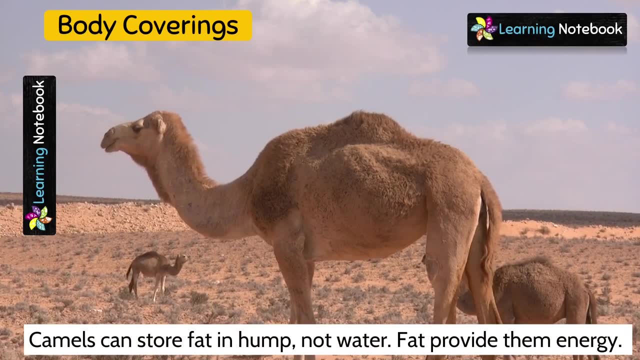 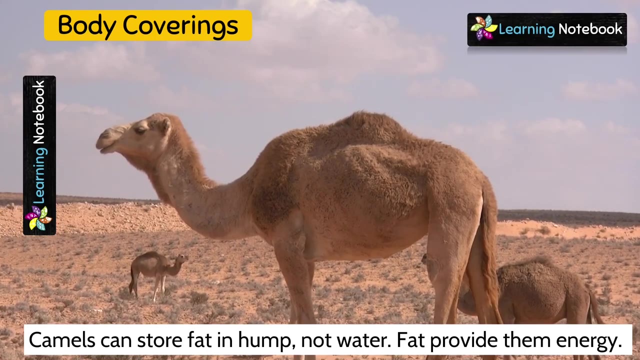 So this is another adaptation in the form of body covering. Now let's see adaptation in camels. To survive in their habitat, ie desert Camels can store fat in hump, not water, And fat provide them energy, Like here. this is hump of the camel. 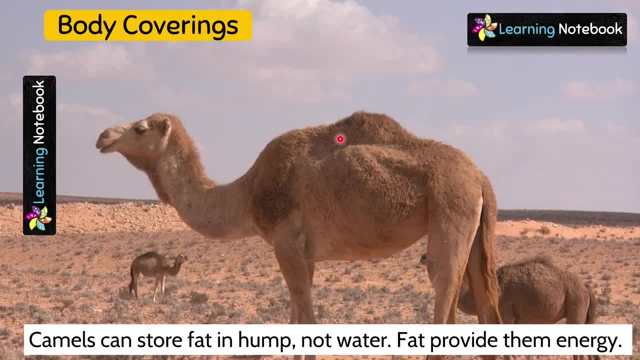 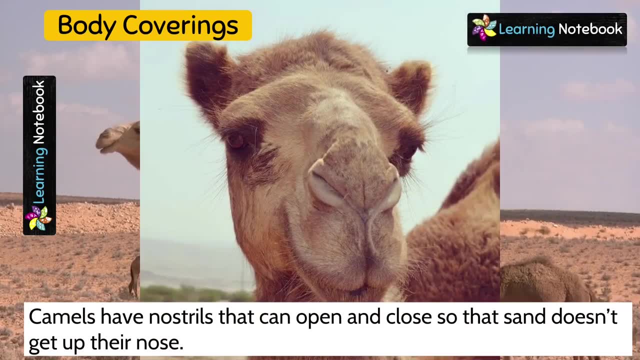 Here it stores fat and not water, And this fat provide them with energy. Camels also have nostrils That can open as well as close. Camels also have nostrils That can open as well as close. Camels also have nostrils That can open as well as close. 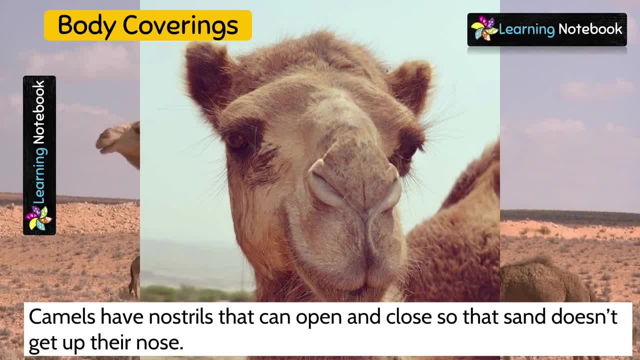 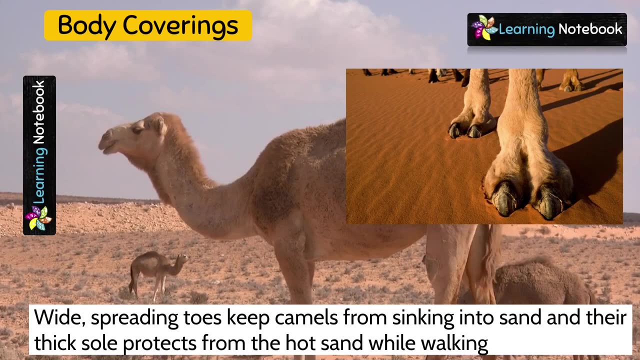 The nostrils are closed when strong wind blow so that sand does not get up their nose. Then camels also have wide spreading toes Which keep camels from sinking into sand And thier thick soul protects them from the hot sand. And their thick soul protects them from the hot sand. 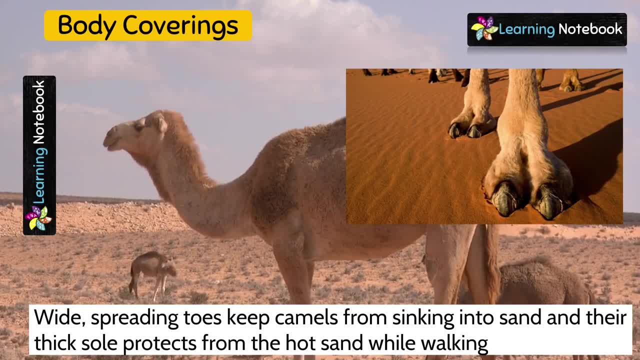 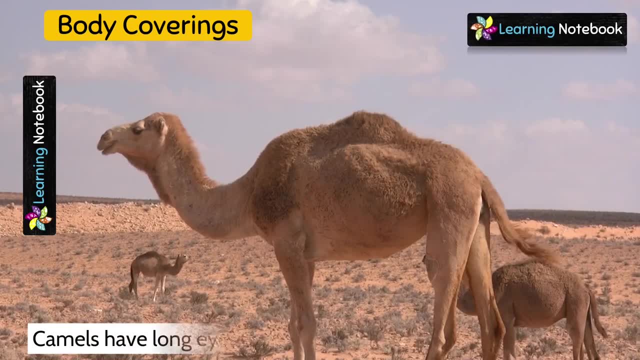 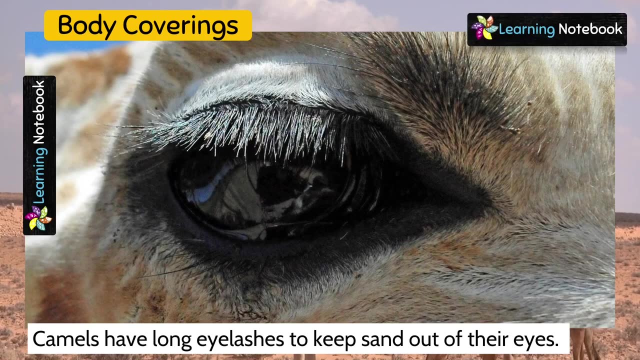 Where is it walking? Look here, these are the wide spreading toes of the camels. Then see, camels have long eyelashes to keep sand out of their eyes. They also have thick eyebrows which shield their eyes from the desert sun. So, students, these body coverings. 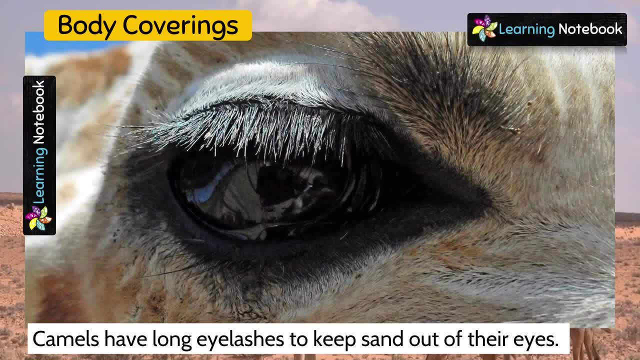 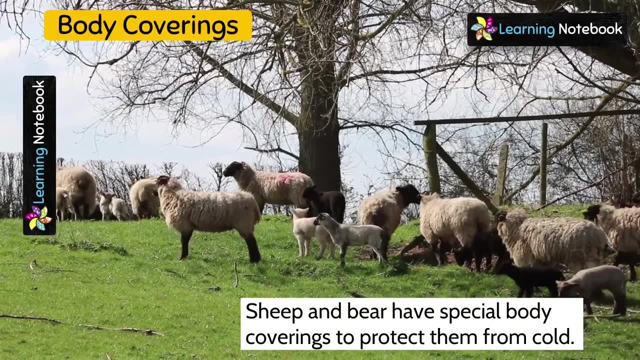 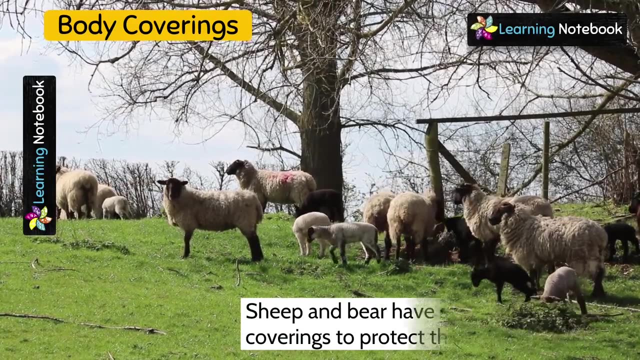 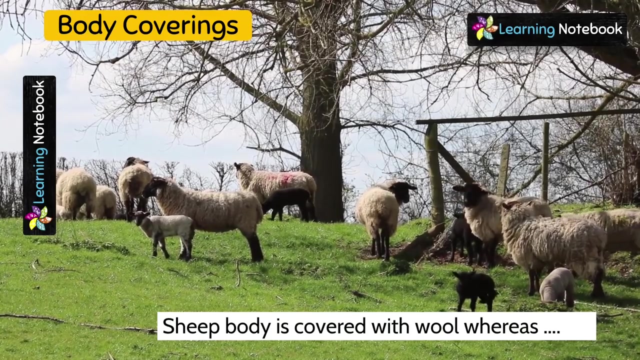 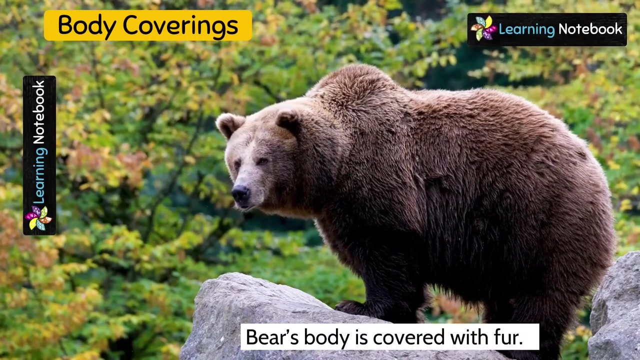 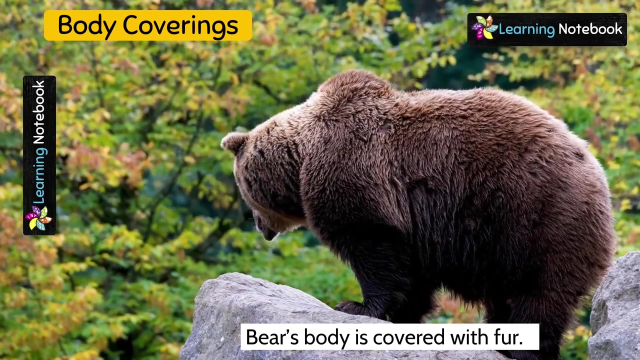 of camels make them well adapted to live in deserts. Next, sheep and bear have special body coverings to protect them from cold. Like sheep, body is covered with wool, as you can see here in this picture, Whereas bear's body is covered with fur. Look here. you can see that the body of bear is covered with. 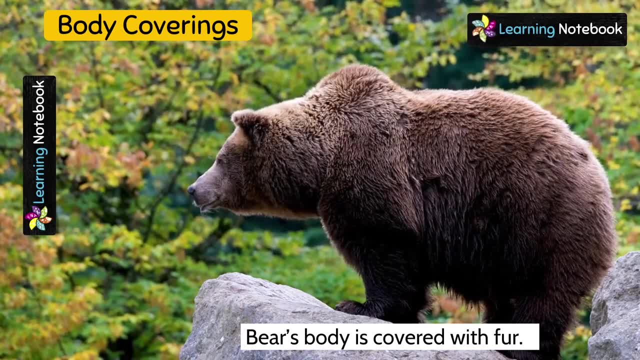 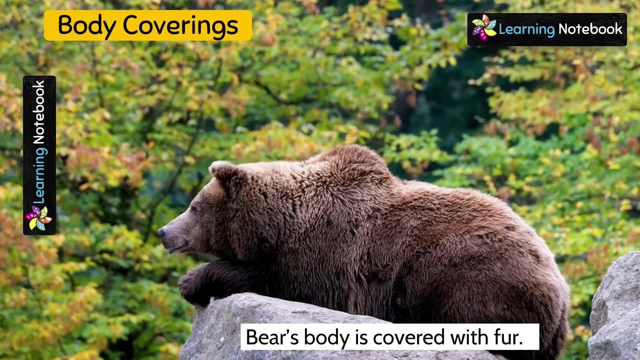 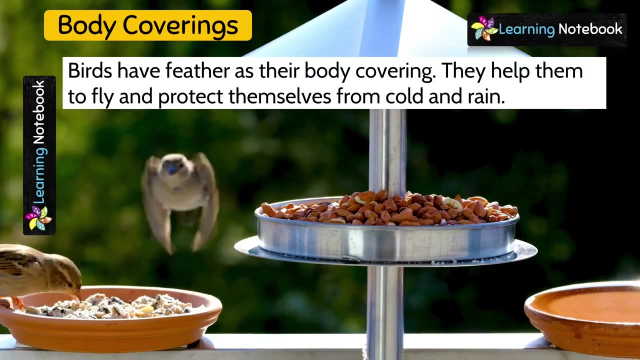 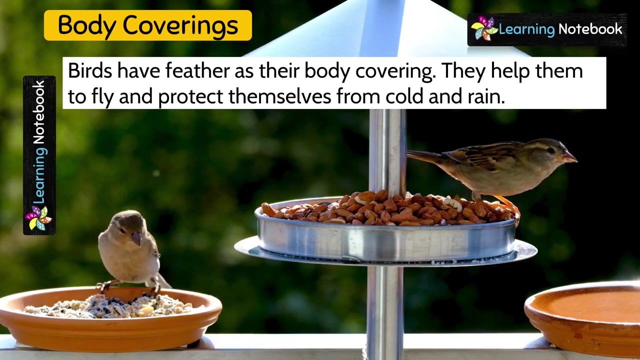 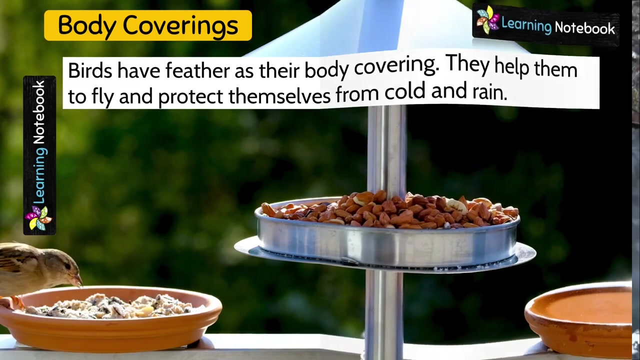 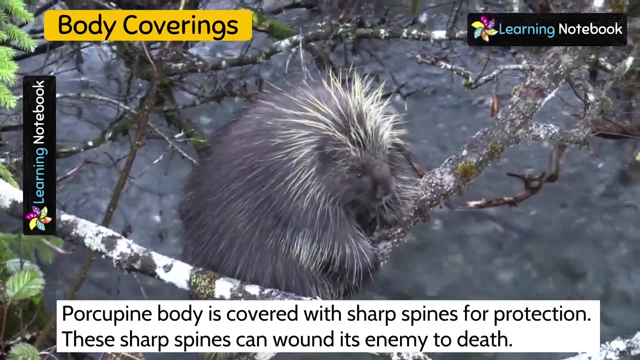 fur, which helps and protect him from cold. Next, let's learn about body coverings of birds. Birds have feathers as their body covering. They help them to fly and protect themselves from cold and rain. Students, this is porcupine. Do you know? body of porcupine is covered with sharp spines. 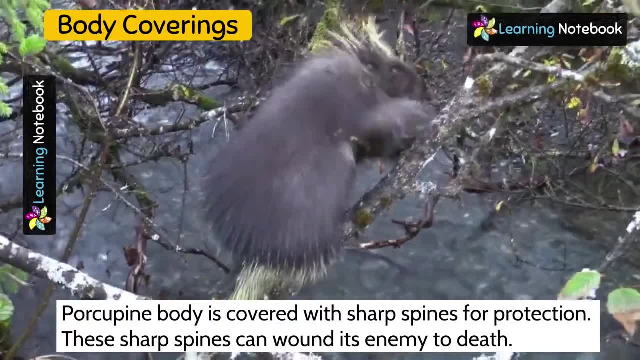 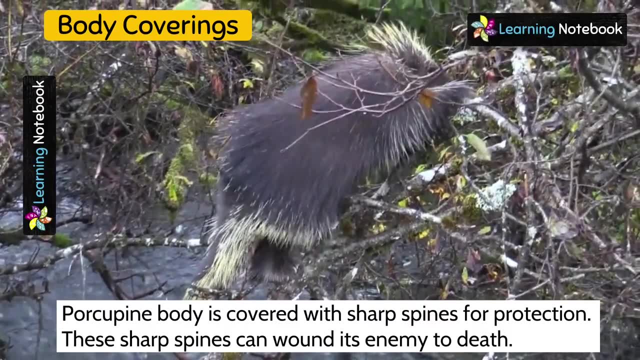 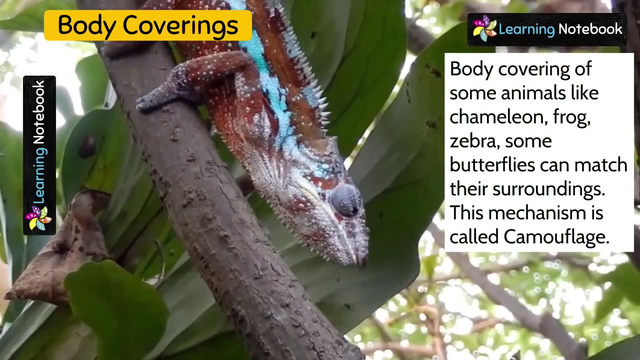 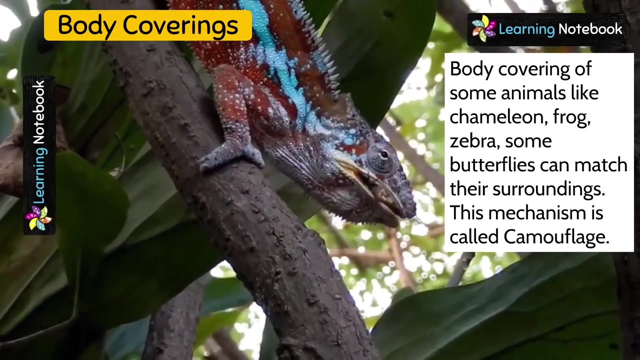 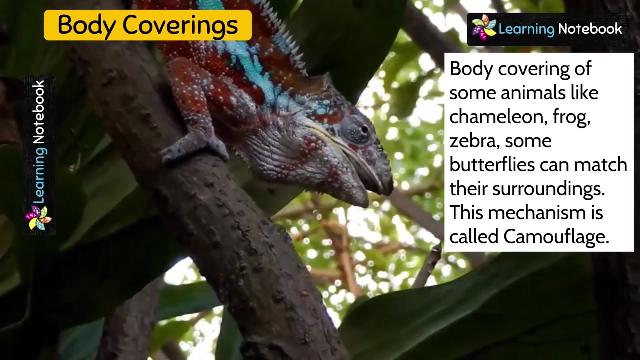 for protection. These sharp spines can wound its enemy to death. So let's learn about body coverings of birds, Body coverings of some animals like chameleon, frog, zebra, Some butterflies can match their surroundings. This mechanism is called camouflage Students. camouflage helps in protection. 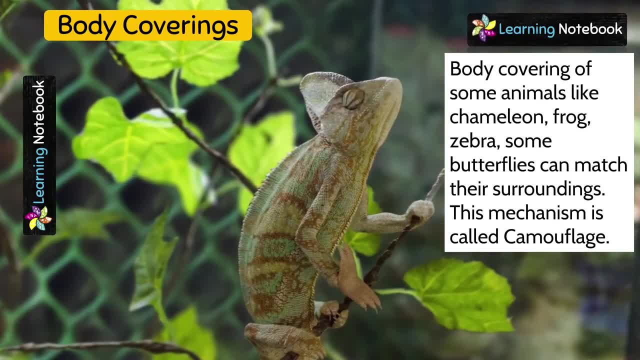 of these animals because it makes animal hard to spot as they get wet or wet. So camels are very protective to animals. I have seen a couple of few camels парung outside me while gathering. They have many wings which are very strong. They are also very hard tomtard to. 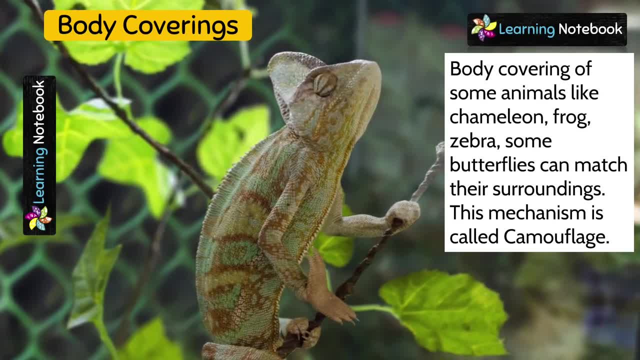 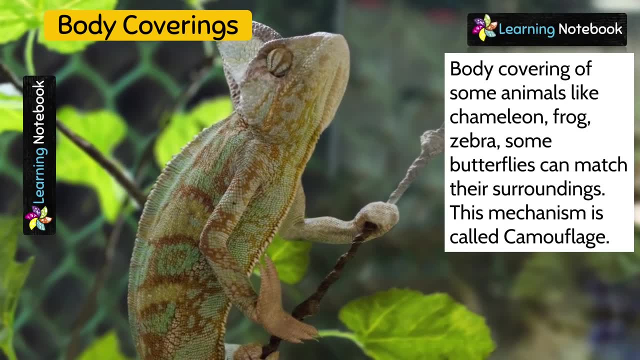 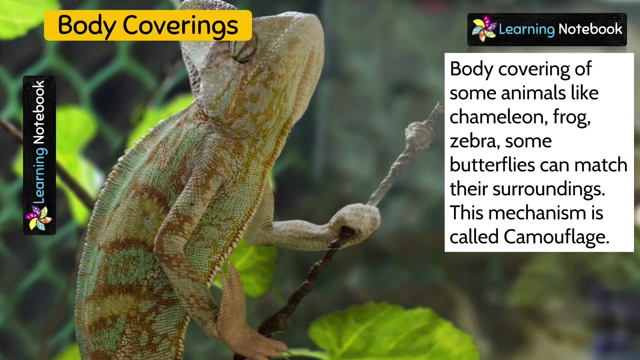 As they get mixed with their surroundings. And do you know, chameleon is even more advanced in this adaptation Because it can even change its body color according to its surroundings. So this was all about adaptation in body covering. Now let's learn adaptation in breathing organs. 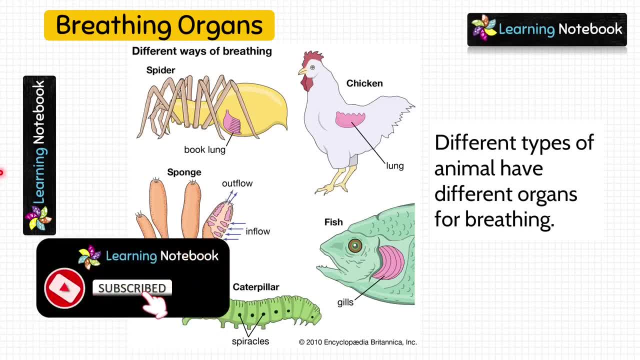 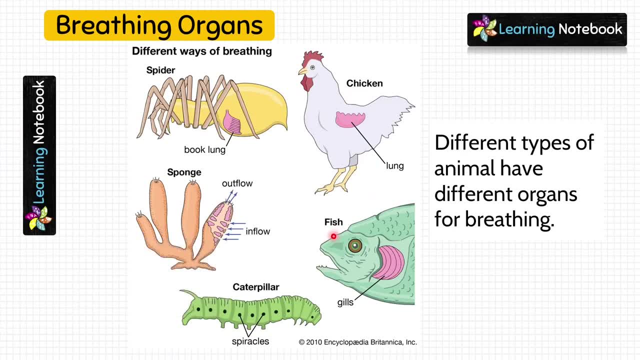 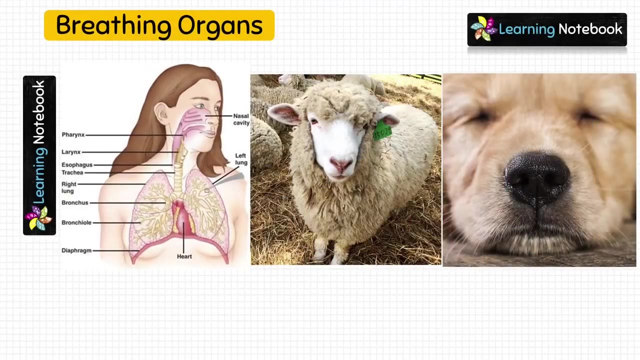 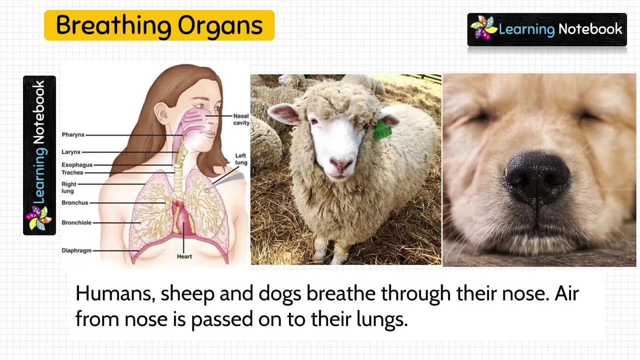 Different types of animals have different organs for breathing. Like chicken has lungs to breathe, Fish has gills for breathing, Whereas caterpillar has spiracles to breathe. So animals have Different organs for breathing. Whereas humans, sheep and dogs breathe through their nose, 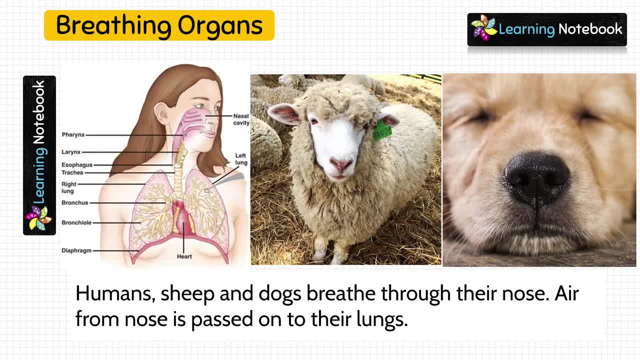 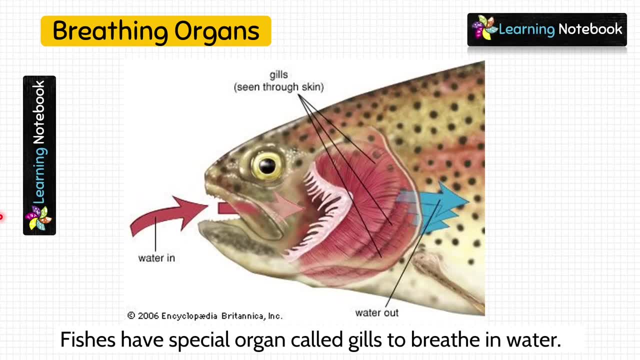 Air from their nose is passed on to their lungs. Students, as I just told you, Fishes have special organ called gills To breathe in water. Look at this picture. Here water goes in And from here water comes out, through gills. 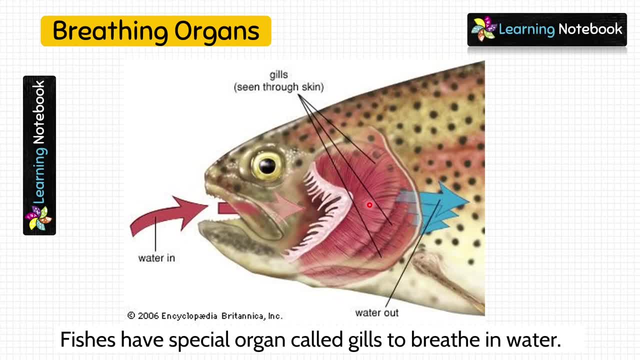 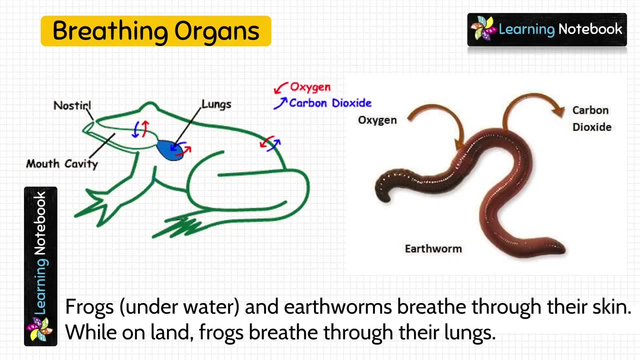 And from this water oxygen is absorbed to breathe. So that's how fishes adapt to live in water: Frogs, Frogs, Frogs, Frogs, Frogs, Frogs when underwater, and earthworms breathe through their skin. Yes, you heard it, right, students? 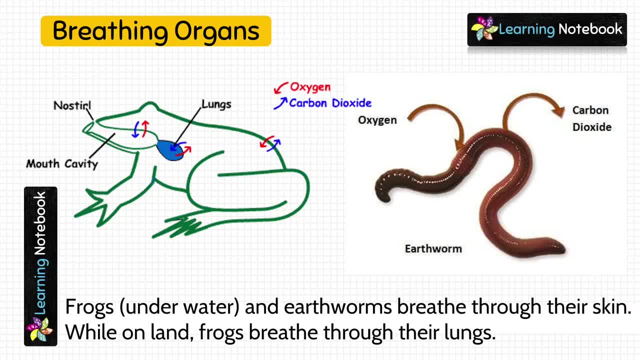 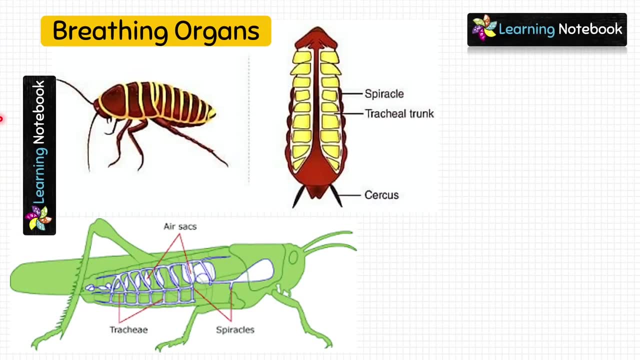 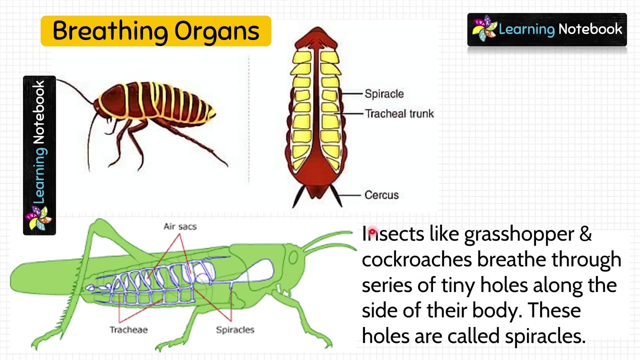 Frogs, when underwater, and earthworms. Both of them breathe through their skin, But frogs, when are on land, They breathe through their lungs- Lungs- Lastly, let's learn about breathing. Insects like grasshopper and cockroaches breathe through a series of tiny holes which are present along the side of their body. 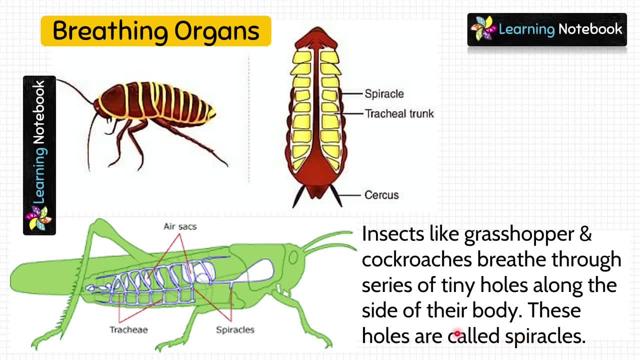 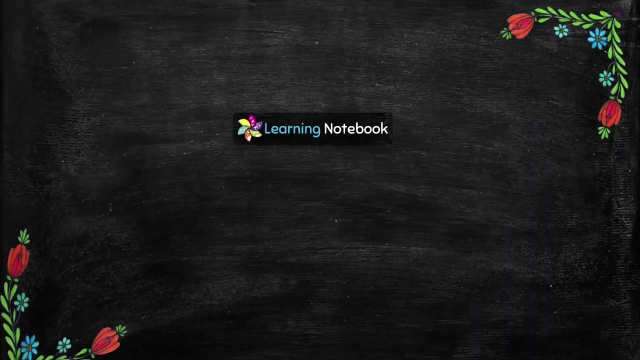 These holes are called spiracles. Like here, These are the spiracles. These are present along the side of body of these insects. So, students, this was all about adaptation in breathing organs. Now let's learn about adaptation in organs for movement. 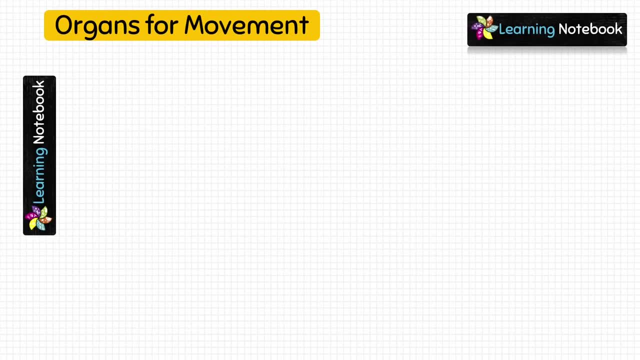 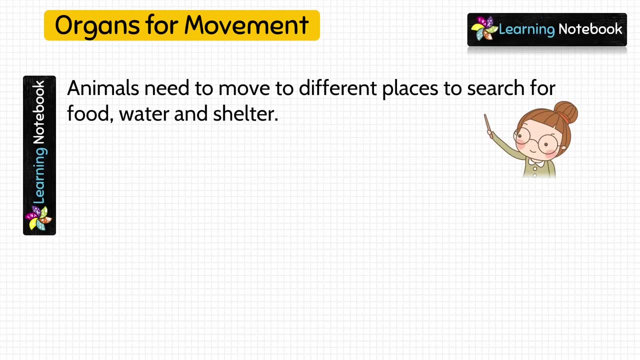 Now let's learn about adaptation in organs for movement Students why animals need movement. Why do they need to move? Animals need to move to different places to search for food, water and shelter. They also need to move to escape from their enemies. 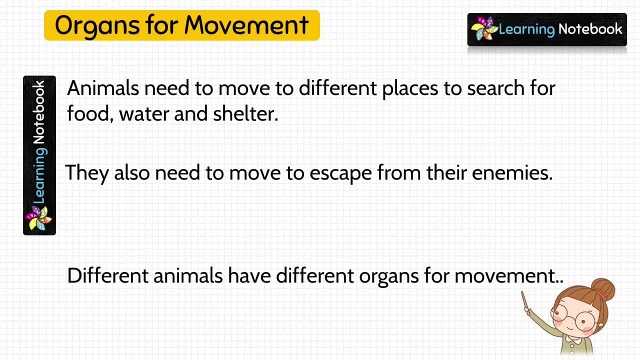 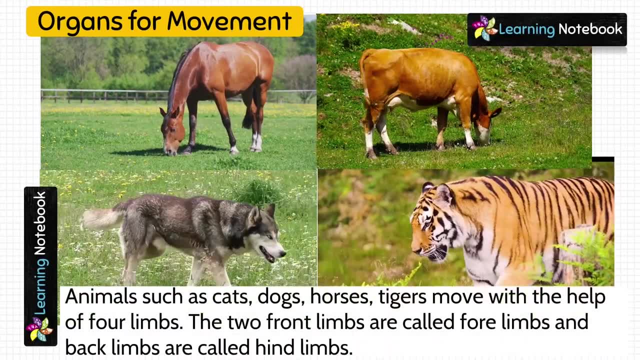 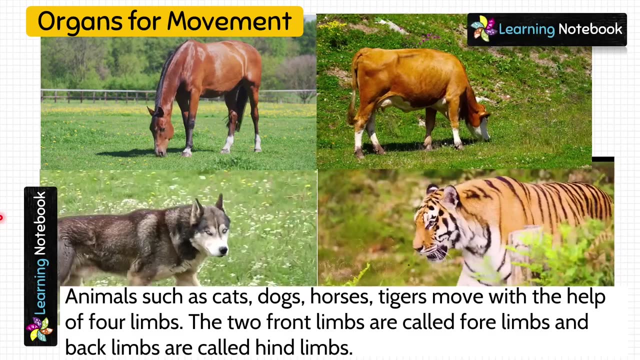 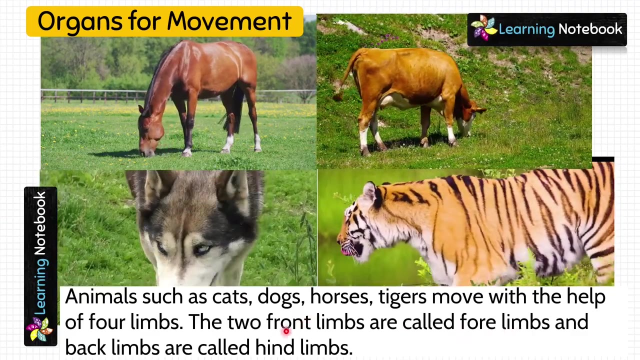 Different animals have different organs for movement. Let's learn about them. Animals such as cats, dogs, horses, tigers. They move with the help of four limbs. The two front limbs are called four limbs And back limbs are called hind limbs. 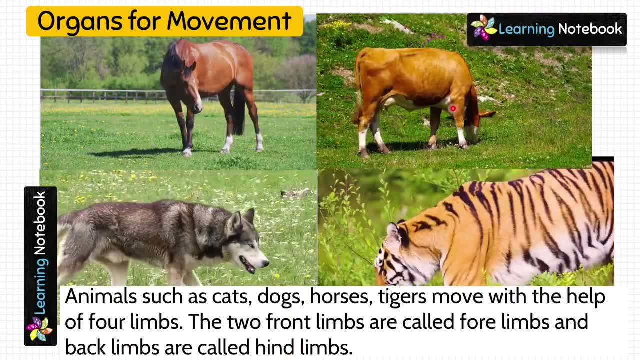 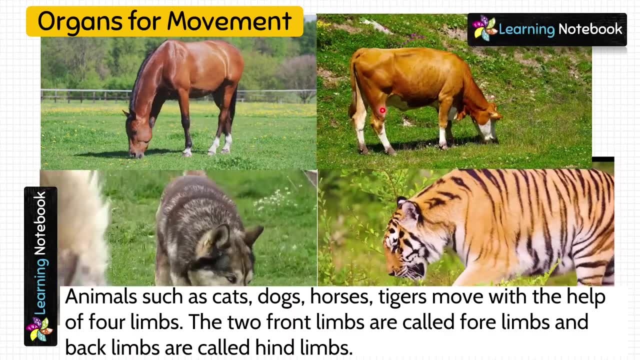 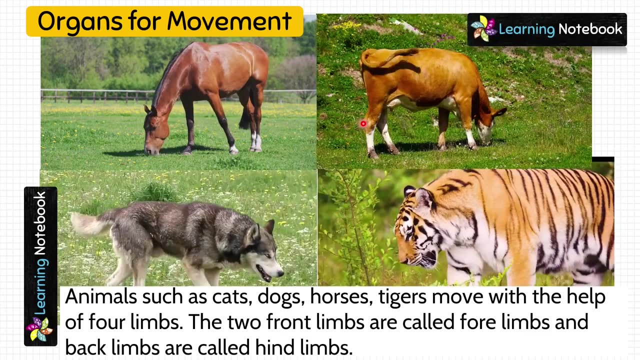 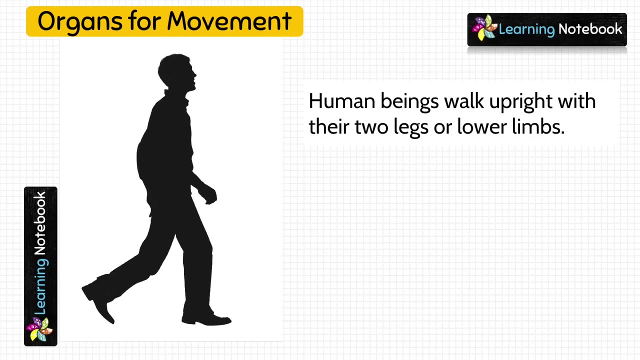 For example. look here, These are the front limbs, So these are called as four limbs, And these two are back limbs And they are called as hind limbs. Similarly, human beings: they both have four limbs. Similarly human beings: they walk upright with their two legs. 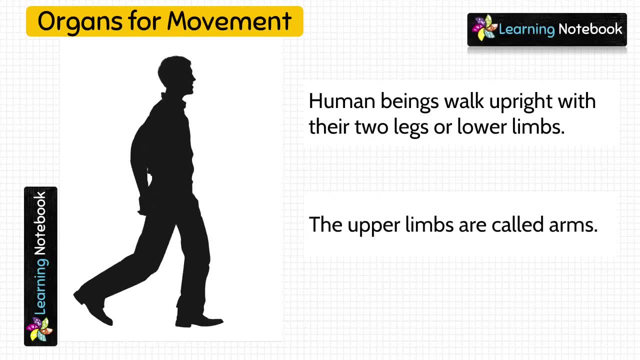 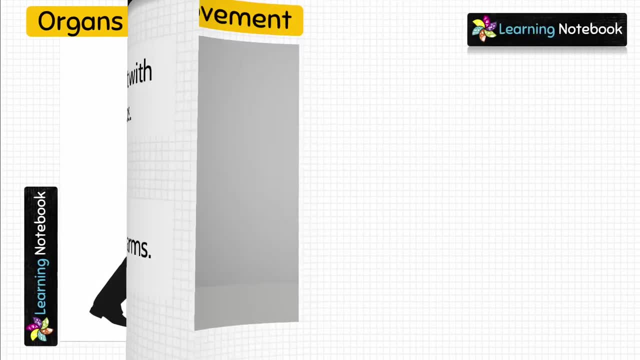 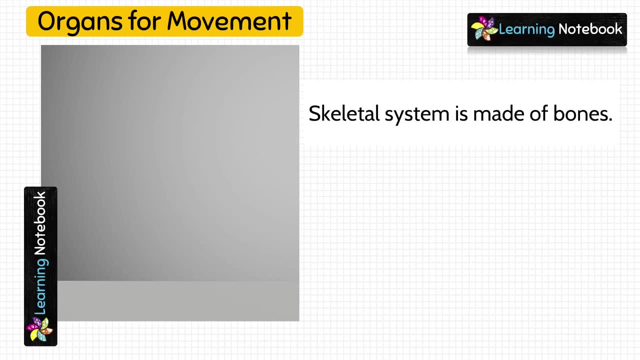 Or legs, are called as lower limbs And the upper limbs of human beings are called as arms. In human beings skeletal system is made up of bones And muscular system helps in all kinds of movement And the upper limb helps in all kinds of movement in human beings. 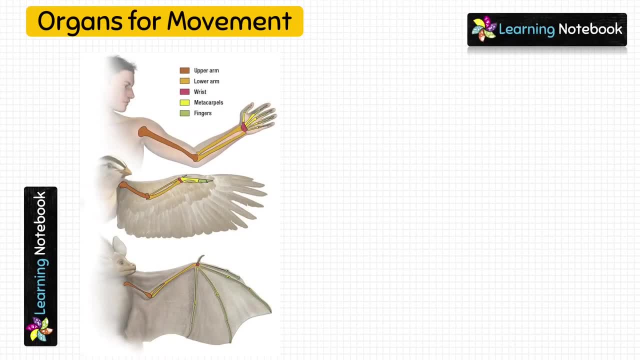 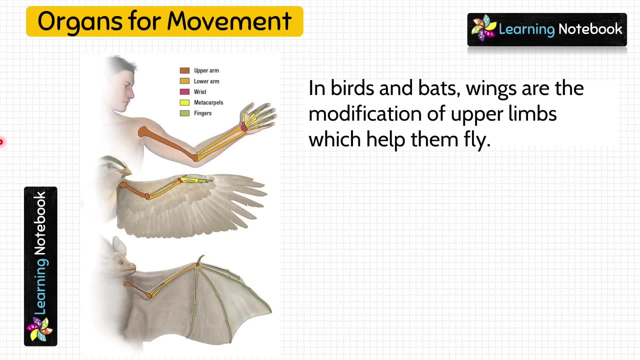 Next is in the human body, in how we can use the moving structure. In birds and bats there are few adaptations Which help them in their movement. For example, in birds and bats, Wings are the modification of upper limbs Which help them to fly. 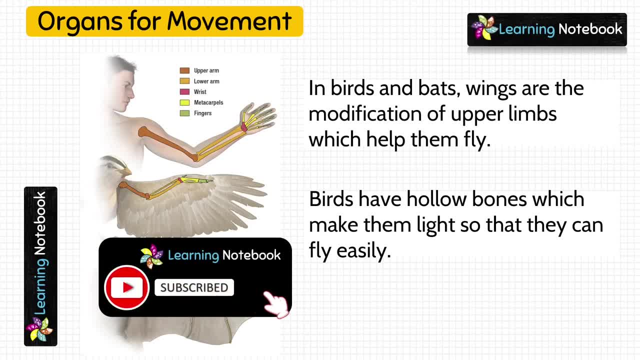 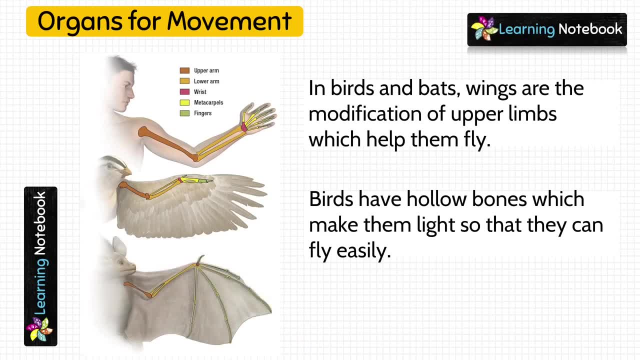 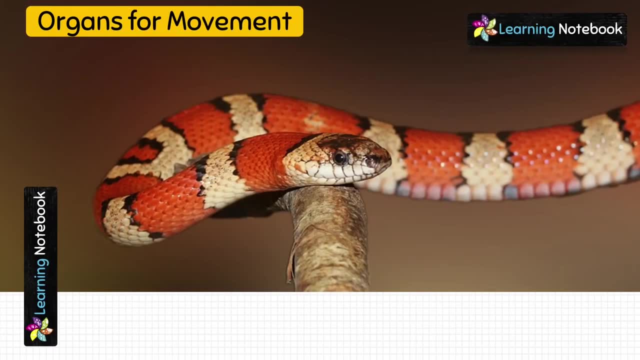 Also birds have. Birds have hollow bones which make them live so that they can fly easily. So these are the few adaptations in birds which help them in their movement. Snakes do not have limbs, So students do you know how do they move? 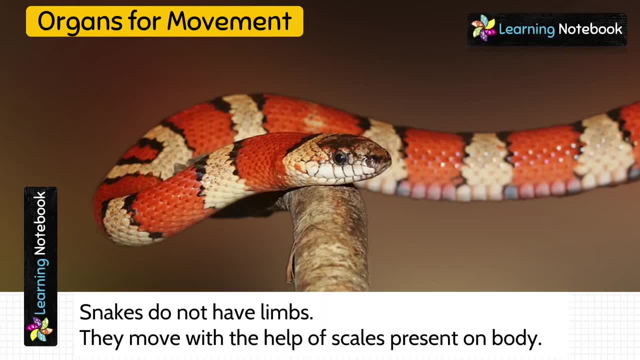 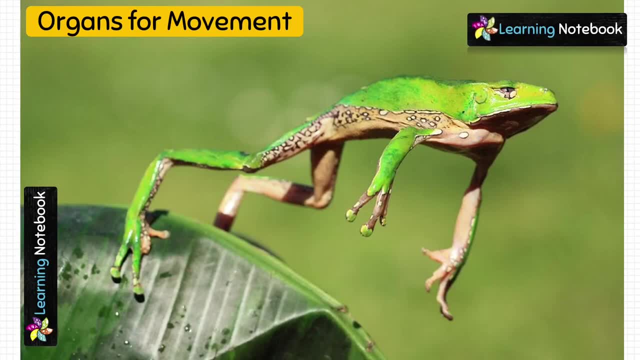 They move with the help of scales present on their body. Next, let's learn about adaptations in frogs for movement. Frogs can hop and jump to a great distance using their strong and long hind limbs. These are the two strong and long hind limbs of frog. 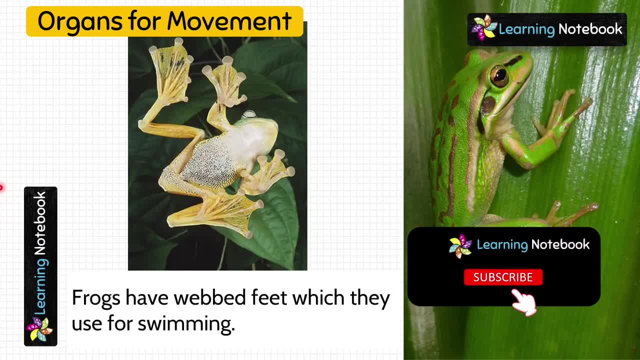 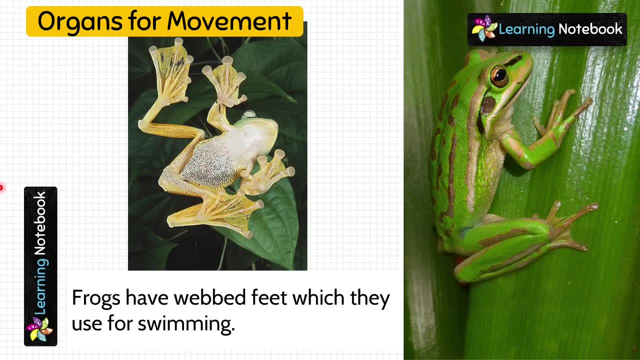 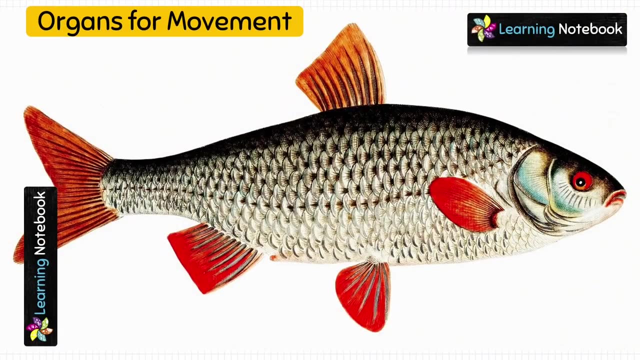 Also frogs have webbed feet which they use for walking Swimming Students. can you tell me which other animals have webbed feet? Do let me know in the comment section. Next, fishes, whales, dolphins. They have special structure called fins on their body which help them to swim in water. 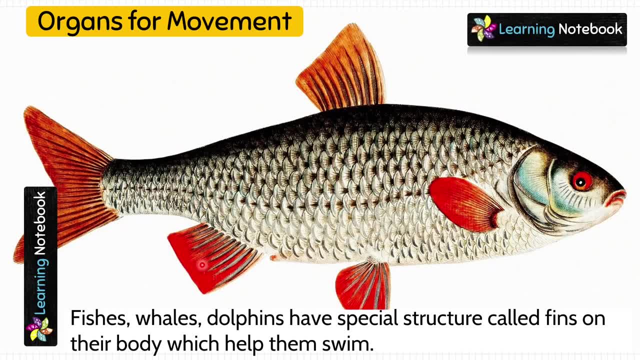 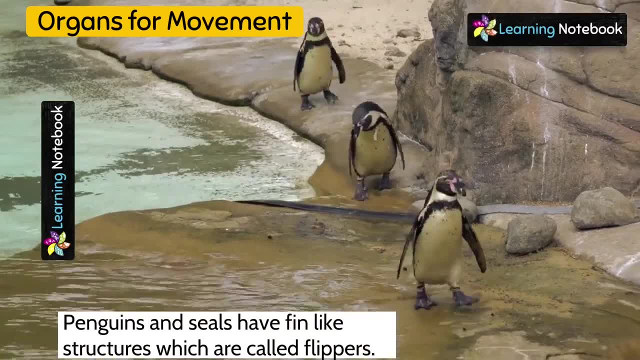 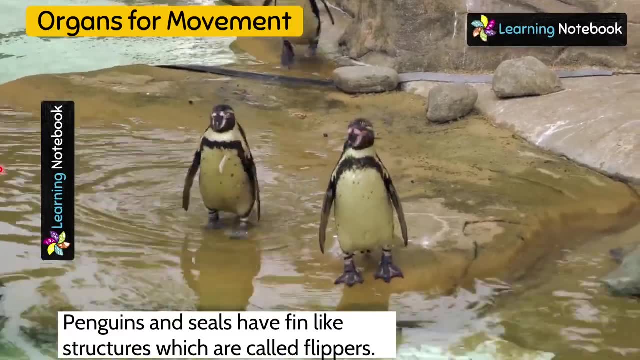 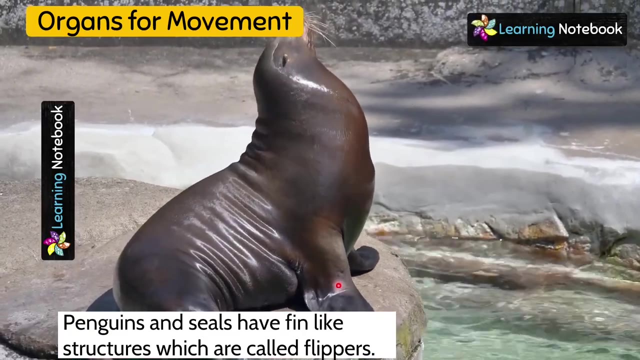 These are the fins. You can see Fins on this fish here. Lastly, penguins and seals have fin-like structures which are known as flippers. These are the flippers in penguins. Now look here. These are the flippers in seal. 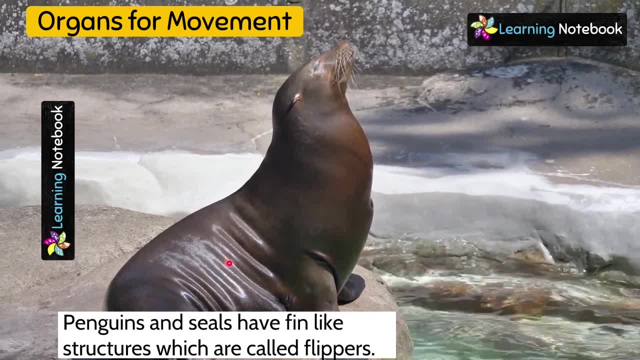 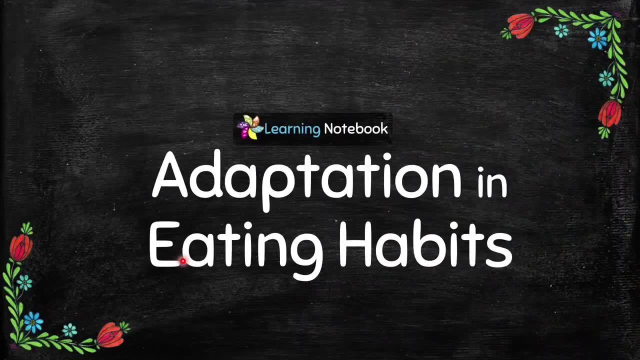 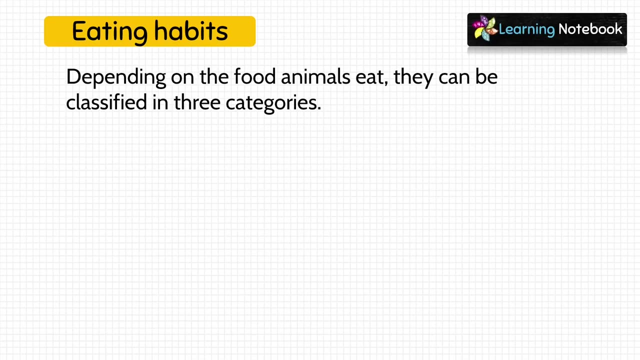 So, students, this was all about adaptations. Now let's learn about adaptation in organs for movement. Now let's learn about adaptation in eating habits of animals. Depending on the food animals eat, they can be classified in three categories. First category is herbivorous animals. 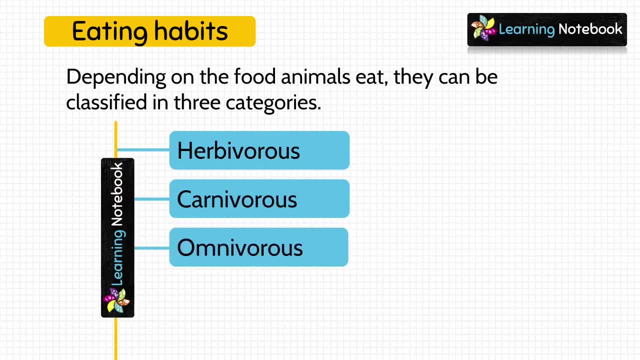 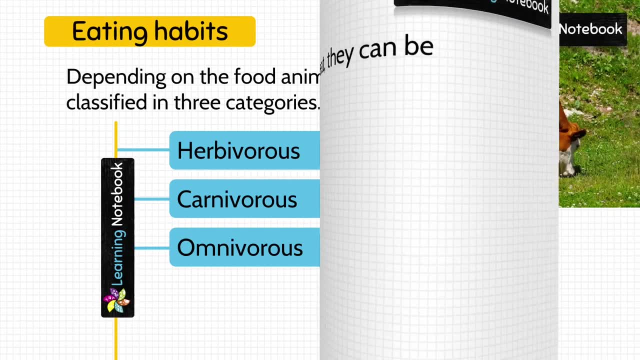 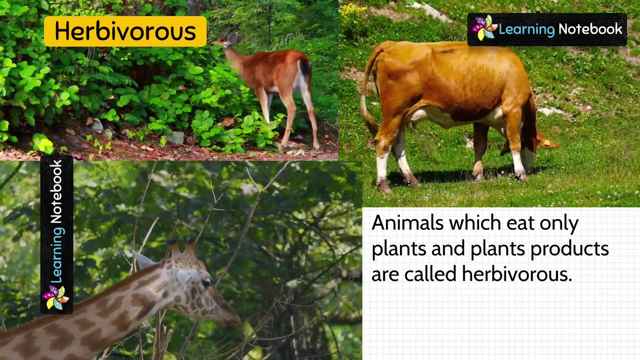 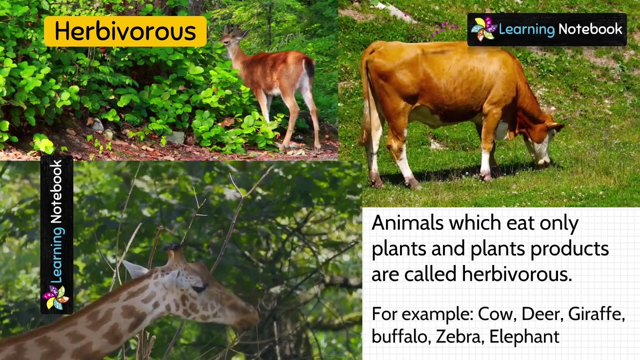 Second, carnivorous animals And last category is omnivorous animals. Let's understand each of them one by one: Animals which eat only plants and plants products. Such animals are called as herbivorous animals, For example, cow, deer, giraffe, buffalo, zebra, elephant.